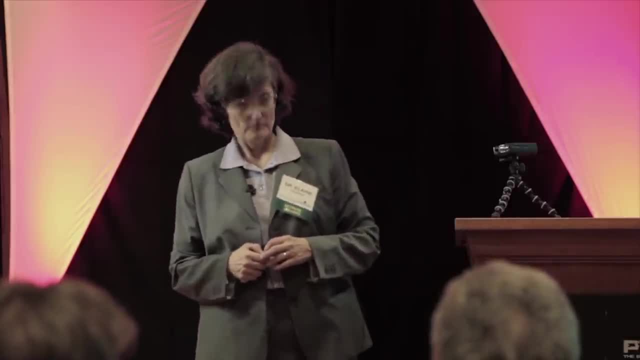 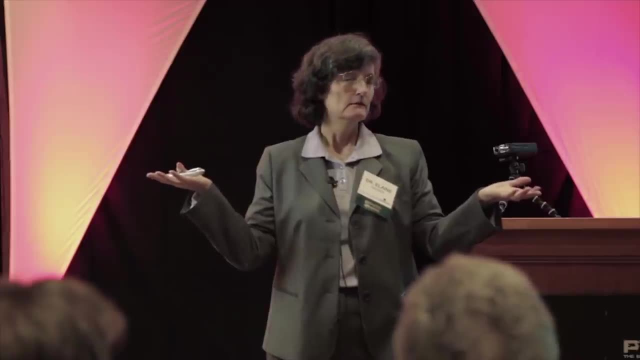 good compost, But if I- and so I need to inoculate my compost pile, they don't come from nowhere. so, Ooh, where do the organisms in your compost come from? No, Most microorganisms don't float through the air, Sorry. In soil. I'm sorry. Where do the organisms in your pile come from? On the surfaces of the organic matter you're putting into the pile? So do you make your compost pile out of straw and manure? How many kinds of organisms in straw and manure? There's a lot, but you're missing. 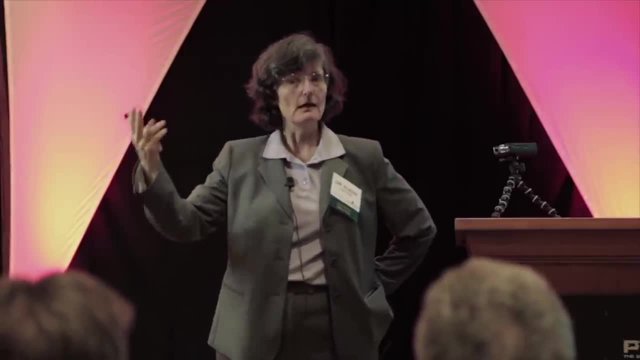 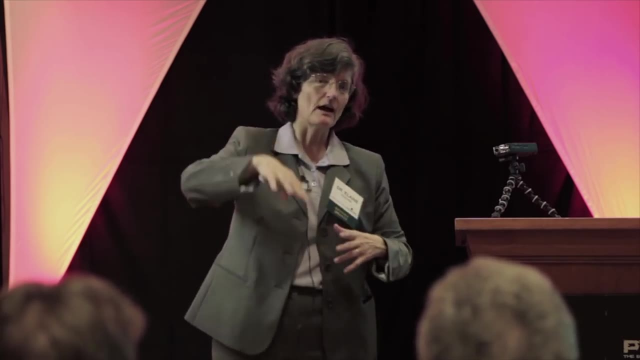 some, Probably about 90%. So let's put some potato waste in there, Let's put some carrot waste in there, Let's put some lettuce, Let's put some- You know all these different kinds of food resources. Let's get some wood chips in there. And do you make wood chips just out of pine? No, You need all the different kinds of wood chips you can possibly find All those different food resources, All the organisms that are living on the surfaces of all those different kinds of foods. Up your diversity The more. 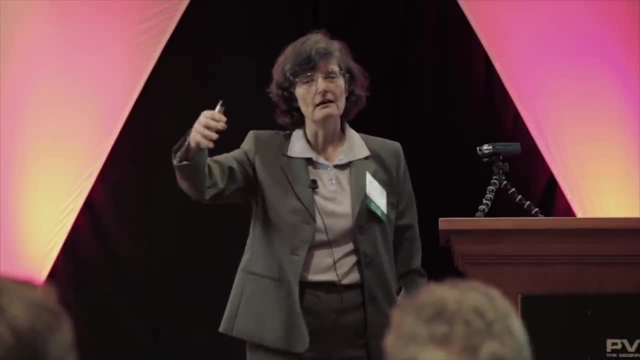 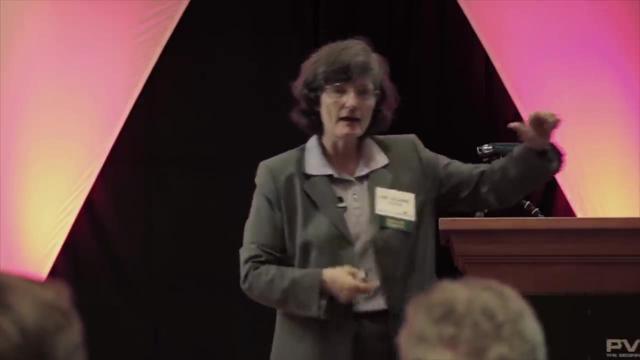 kinds of foods, the more inoculum you're getting in there. And what if you think that maybe the stuff that you're getting doesn't actually have the fungi in there? Then take a hike out into an old-growth forest and dig down to the O horizon, the interface between the O. 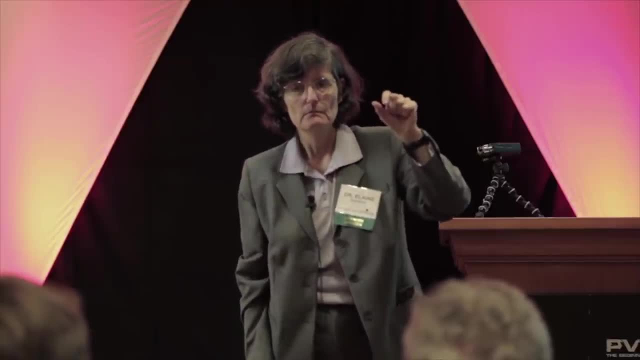 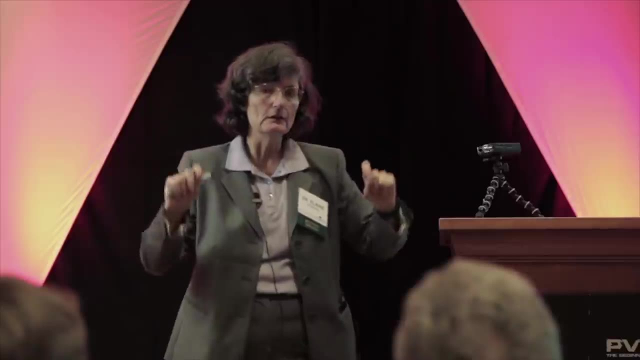 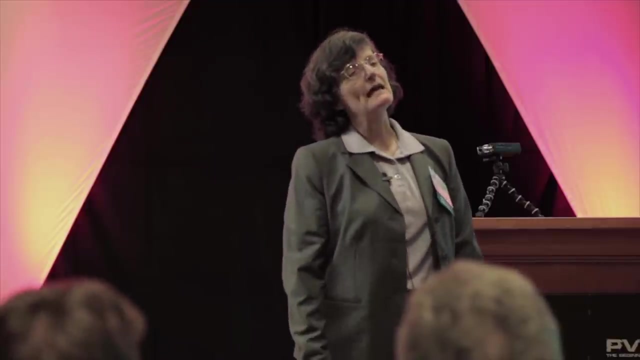 and the A horizon and take a teaspoon- No more than a teaspoon- because we really don't want to destroy our old-growth forests, okay, So be gentle, be careful. For the rest of your life, you will never go on vacation, ever again. Instead, you're going to be taking. 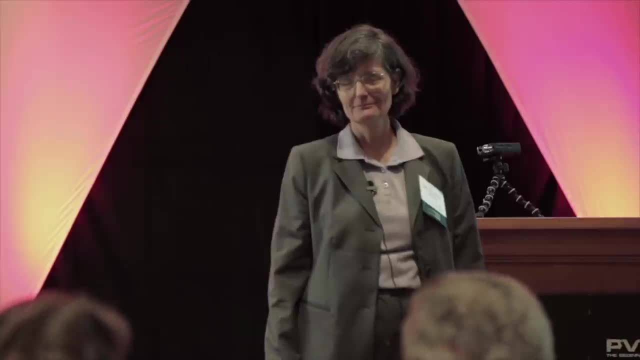 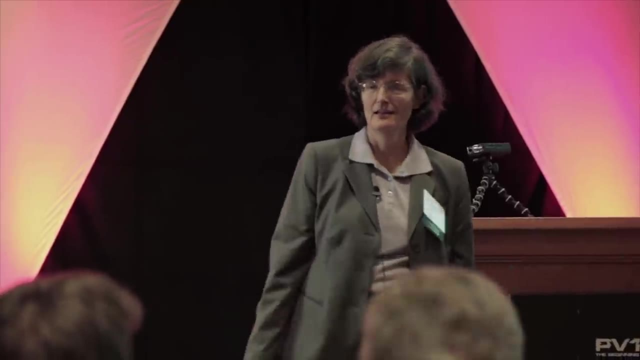 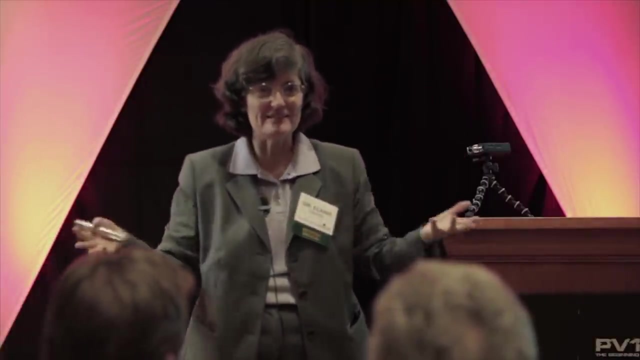 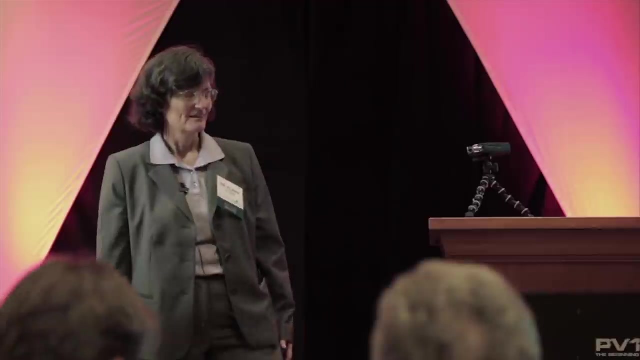 an organism-collecting trip. It's a business right off. Come on. You don't think the oil companies don't do exactly the same thing? How about doctors who have their conferences in Vail in December? So why can't we do it? We're going on an organism collect—now. 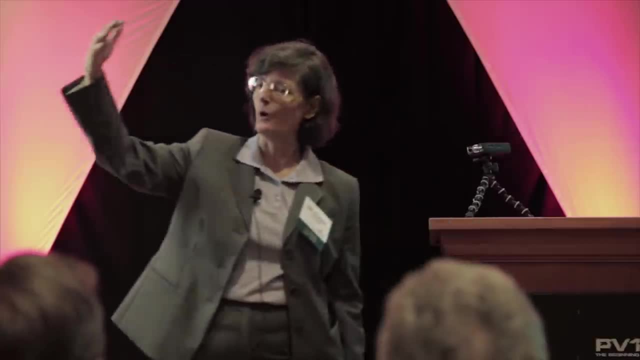 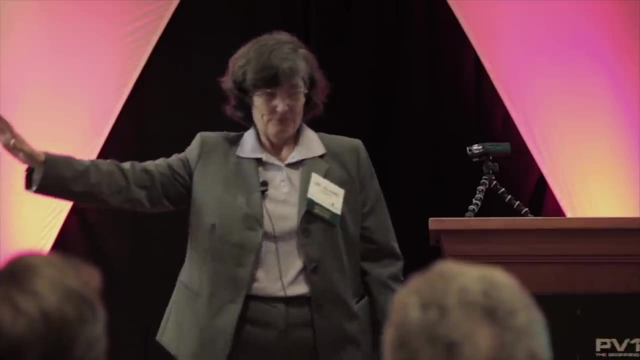 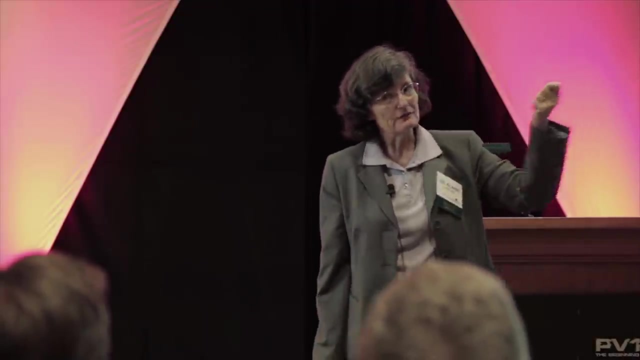 here in Southern California—. are we going to go to Hawaii to collect our organisms? No, probably not going to benefit you too much. Plus, Pele gets mad at you. So are you going to go off to New England to collect your inoculum? Well, you know, if you bring some stuff back from there, most of them are not going to survive here in Southern California, are they? They're not really very used to 120-degree temperatures, no humidity, So you might gain a few things, but you're going to have to make certain you always put it through the composting process. So 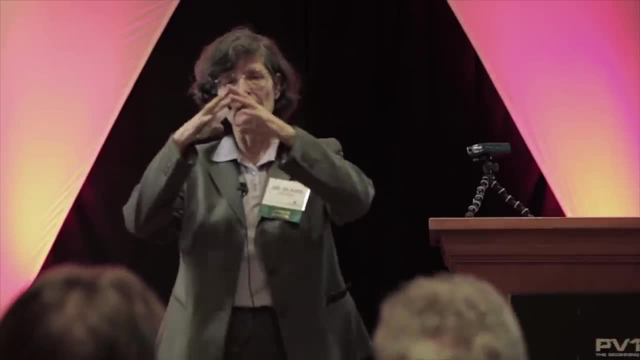 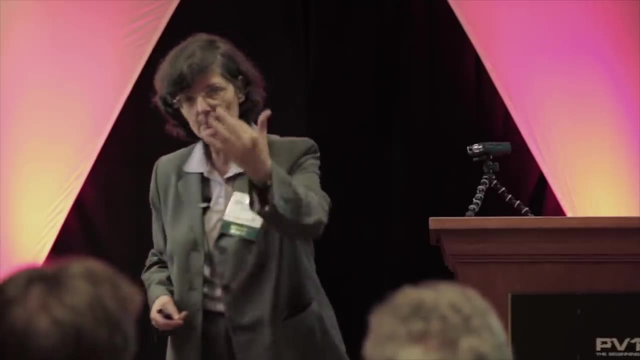 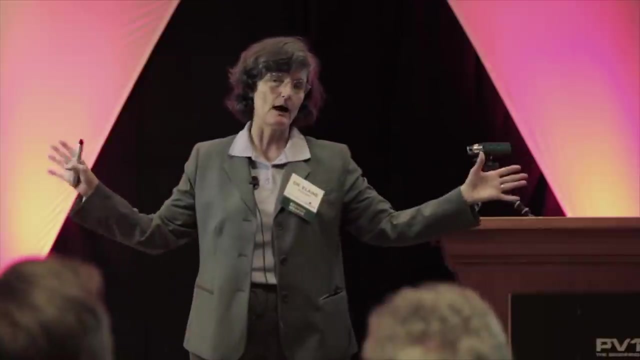 your habitat here. the conditions here wipe out those things that can't grow, that shouldn't be present here. We've got to put things through that composting process so any diseases, any pests, any problem organisms are wiped out in the composting process. So if you can't, 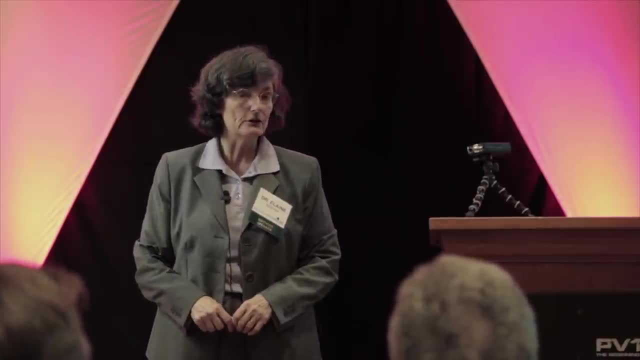 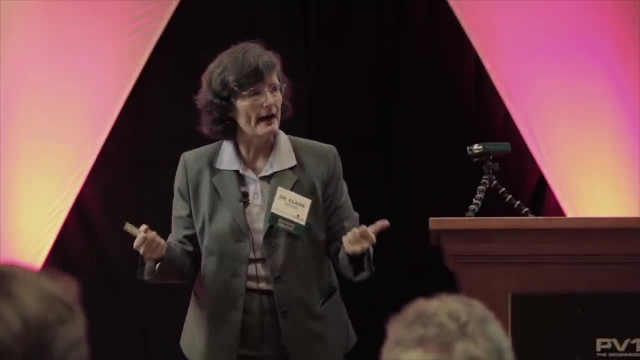 count compost. let me direct you to people who are making really good compost And I would hope that some of you in this crowd would take on the challenge of starting to make really good compost for all of your neighbors. And you know, we drive the municipal composting. 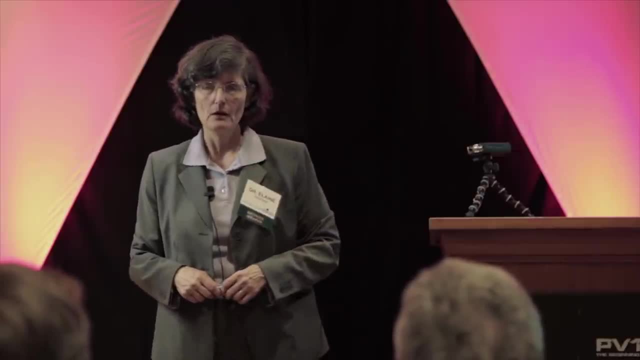 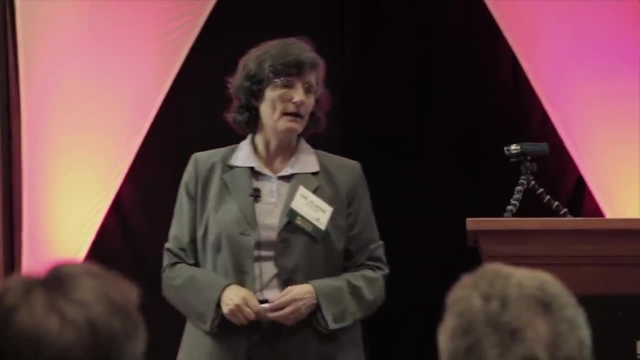 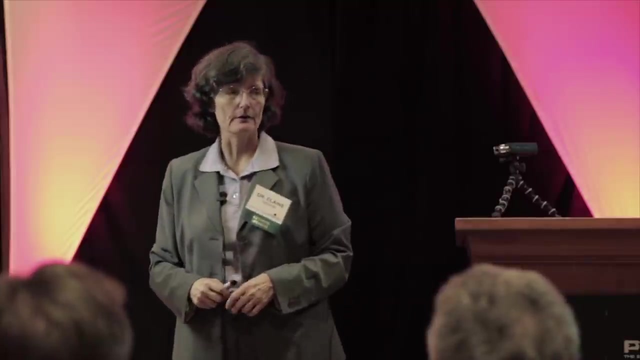 operations—composting operations—municipal reduced waste operations. We drive them out of business because no one should be buying that stuff and believing that it's compost. Okay, there's exceptions, so I can't do across the board, But let me finish this example. 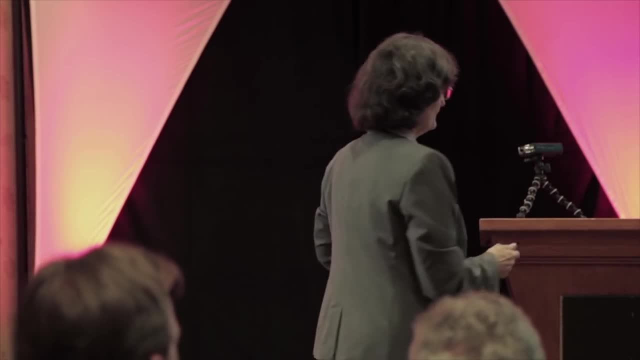 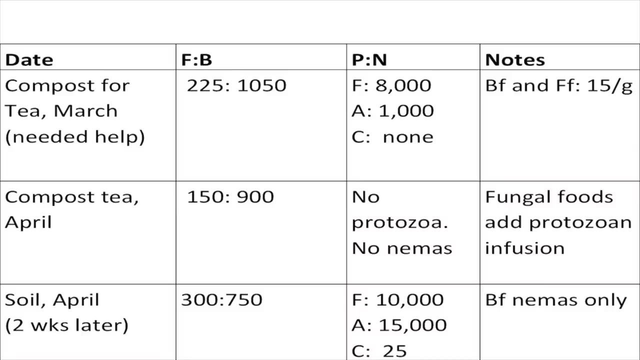 I'm sorry, I keep calling on people and I'm not going to call on any more people until we're done with this example. Okay, So here we are. We've got to do a better job of maintaining our compost through that wintertime period. We've lost some protozoa. We have gained. fungal-feeding nematodes. The nematodes don't like disturbance. If they don't like disturbance, if you turn that pile, if you mix that pile, your nematodes are in there, going. oh my god, it's an earthquake- Run And they're gone. They're not there anymore. So now what? 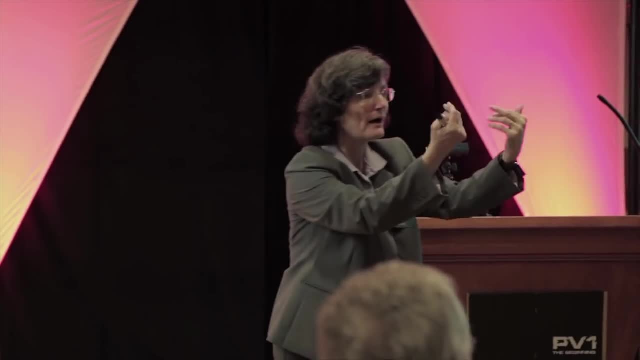 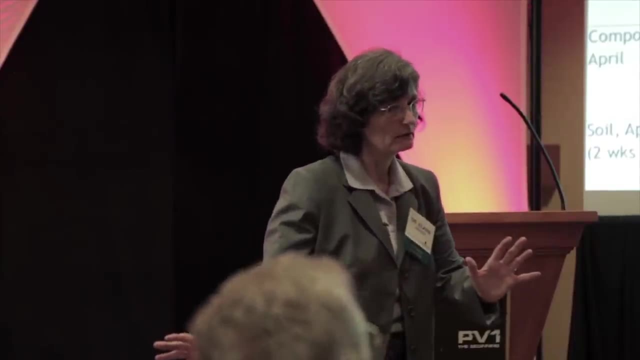 are you going to do to bring them back? You've got to lure them back, Come back, come back. And it takes them a while to say: is it safe? Is it going to happen again? Is there going to be another earthquake? Okay, maybe. And then you turn the pile again: They're gone. 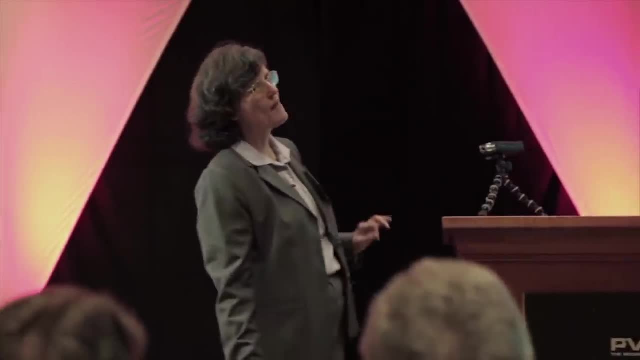 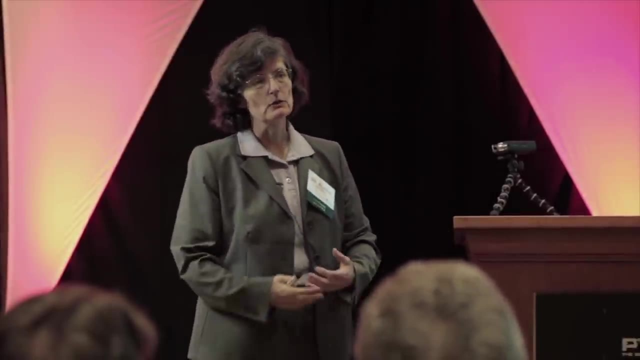 And now they're not coming back because they've learned that you're not trustworthy. So mix, turn the pile to the least amount that you can. So you've got to keep that compost in an area where there's good airflow, where there's good oxygen. You've got to maintain. 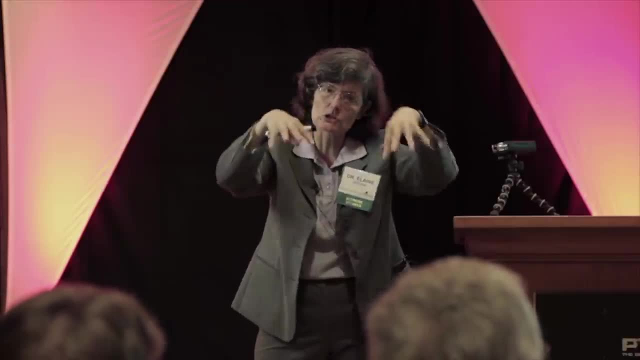 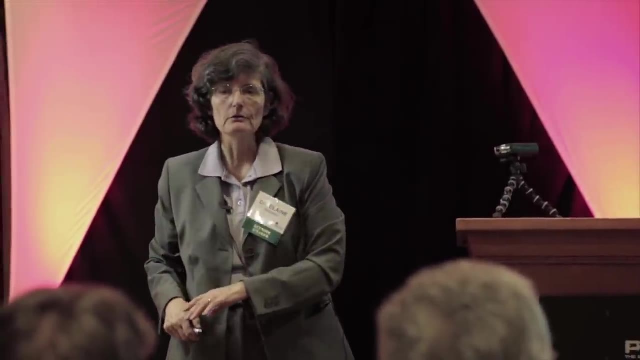 the organisms. so you maintain the structure, so oxygen and water can move into that pile all the way through. You can't let it get water-locked, You can't let it dry out. You've got to maintain it. So generally what I tend to do is I have a little spritz bottle with a little bit of humic acid water. One gallon of my tap water. one drop of humic acid goes into that gallon. So I've got that spritz bottle and when I walk by first thing in the morning I just spritz it Nice light layer, Put the cover back on and it generally stays really nice. 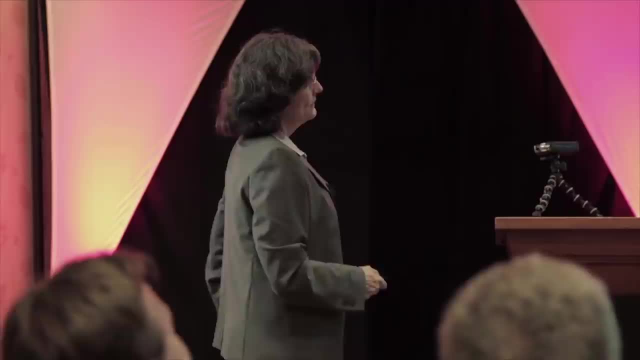 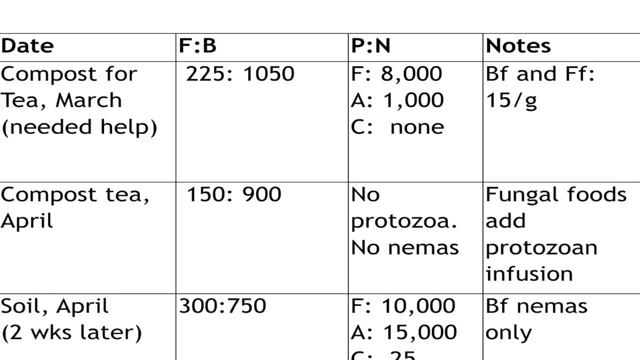 My organisms just get happier and happier. So, unbeknownst to me, they took this compost and they made compost tea from it. Oh yeah, I think there's something wrong with their tea brewer because we had- well, it was nowhere near this bad a ratio in the compost. We've lost more of our fungi than we've lost bacteria. We lost both bacteria and fungi in that tea brewer. This is one of those old micro-brewers and every time the tea passed through the pump it sliced the tea, It sliced and diced the organisms as it passed through the pump. So the numbers go down every. 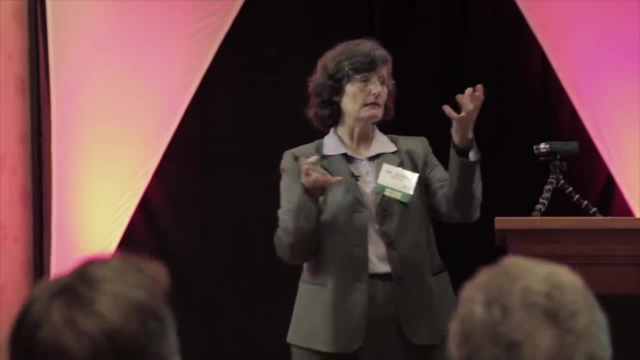 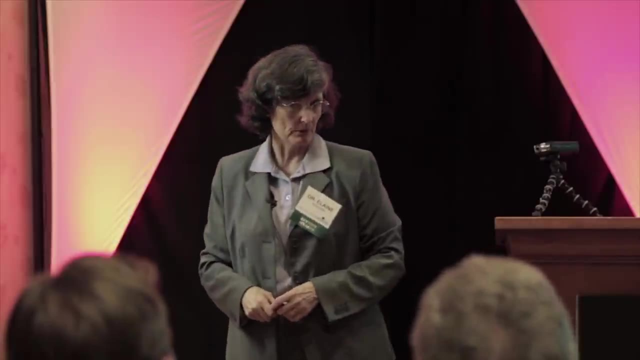 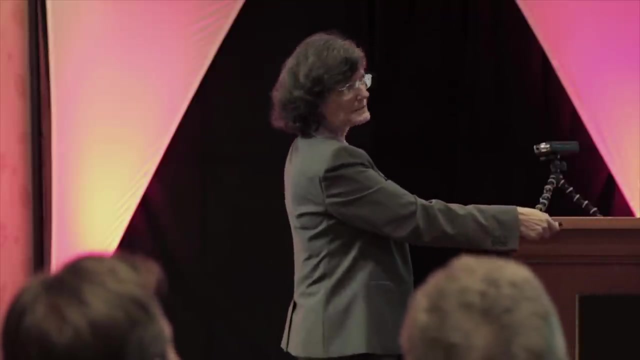 time When you have a tea brewer where the tea is passing through a pump, there is no way to maintain the biology in that tea brewer. So what's the right tea brewer? Come to the class No protozoa. So what else did we lose? So why do you bother putting on a tea like? 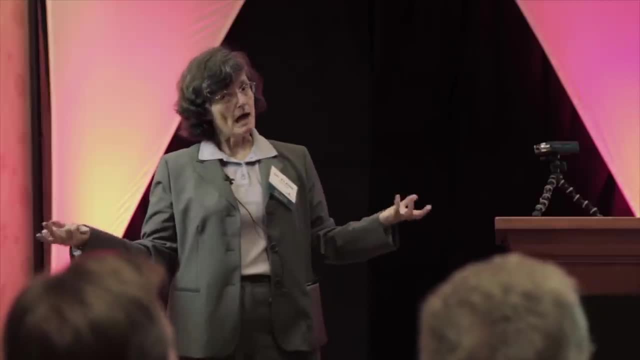 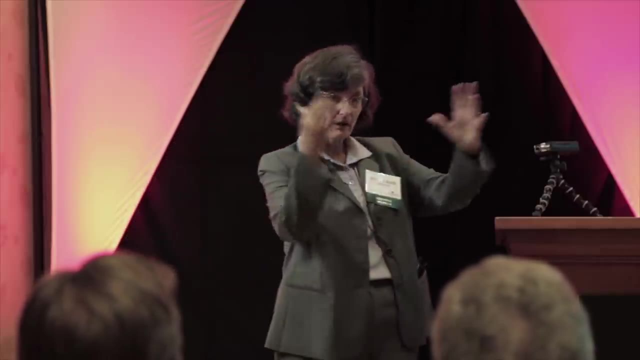 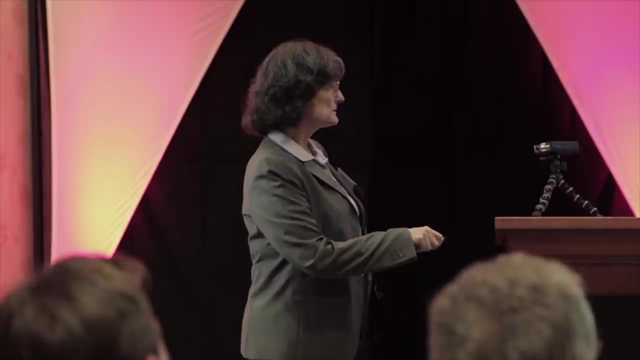 this. What is the point? It's a lot of work. It takes a fair amount of electricity to brew for 24 hours at room temperature or at the ambient temperature and it's not really going to give you the benefit. So when they looked at the soil two weeks after applying that compost tea things. 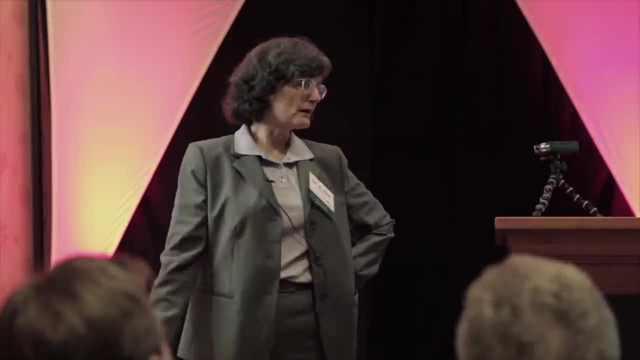 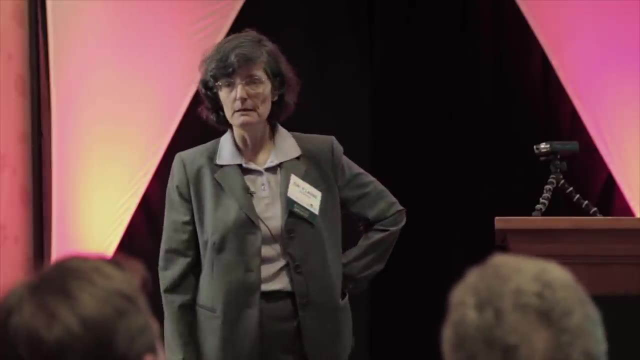 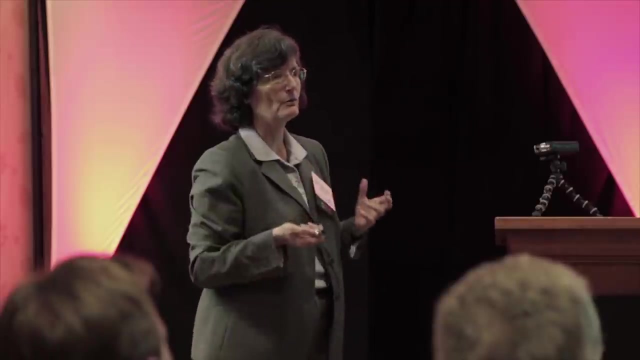 are worse. Things are going the wrong direction. We are not fixing anything. So when we got these data- and we did them all at the same time- it was a lot of work- I was a little upset because a waste of money and a waste of time. We're not going the right. 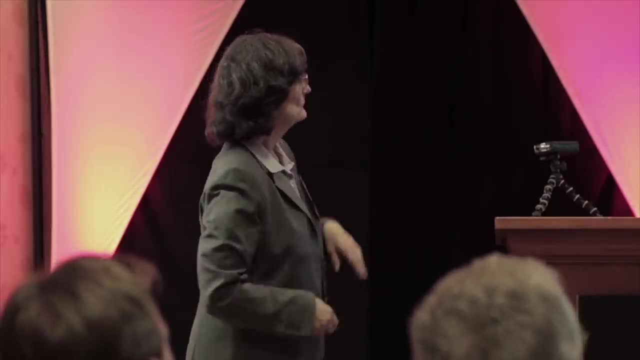 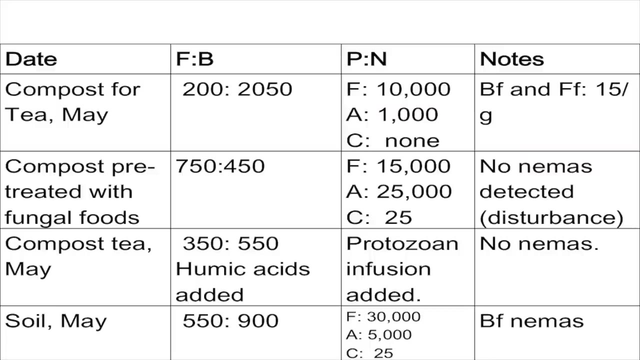 direction. So let's keep going. So here's me. We looked at the compost So I said: add fungal foods. So they added fungal foods. We waited another week for us to apply anything because we had to let those fungal foods bring that fungal flavor back into the soil. So 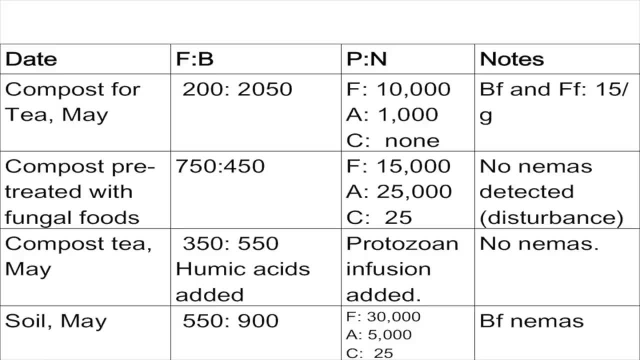 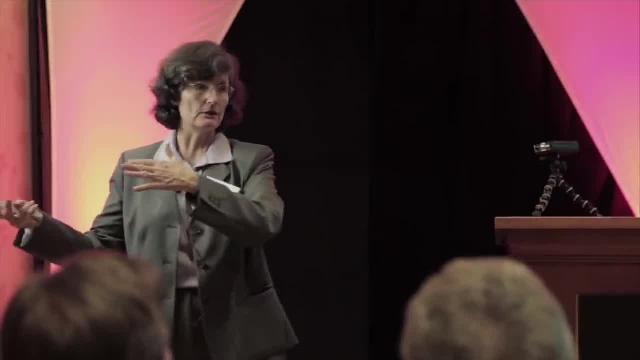 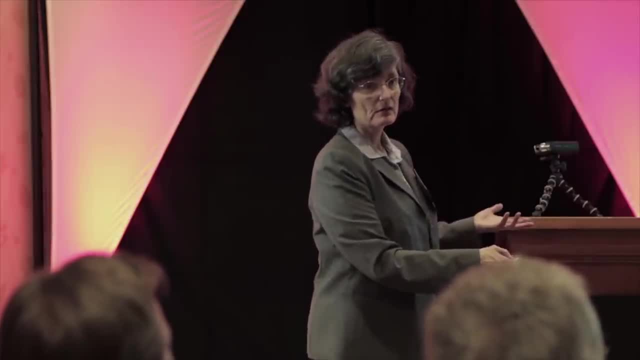 these fungal foods bring that fungal community up to high enough levels. So now look at this: As the fungi grow, they compete with your bacteria Aerobic good guys. But we kind of made our nematodes head for the hills because we turned this in order to add the fungal foods. So 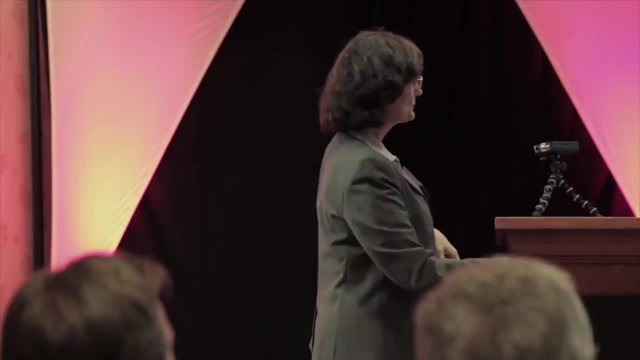 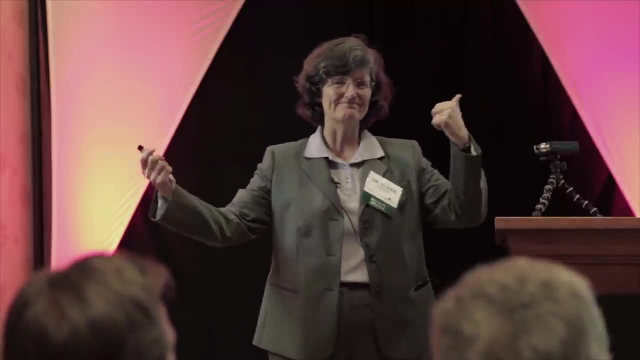 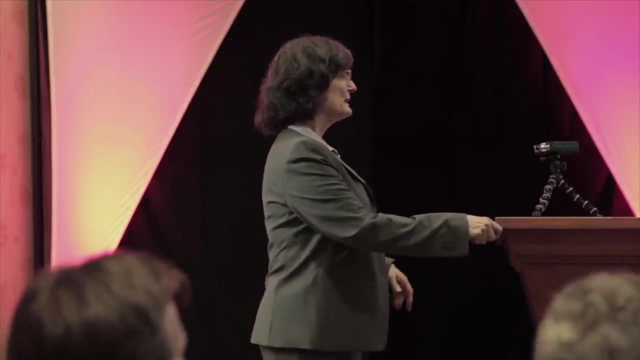 our nematodes went gone, but we improved everything else. So now we make the tea from that. Oh darn, they made it. They made it in the same tea brewer. So we added a protozoan infusion because we had no protozoa in. 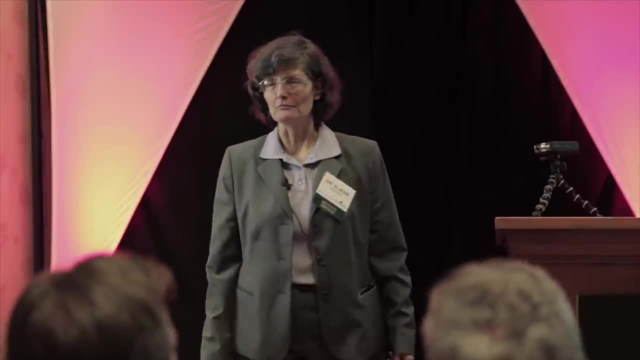 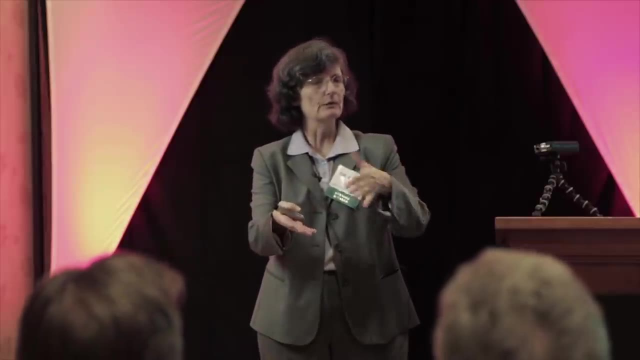 that tea? What the heck is a protozoan infusion. So we're going to take a five-gallon bucket and we're going to put plant material where we know we've got really good sets of bacteria, where we've got really good protozoa. So we've got the phylogenous and the meby in a dormant state And 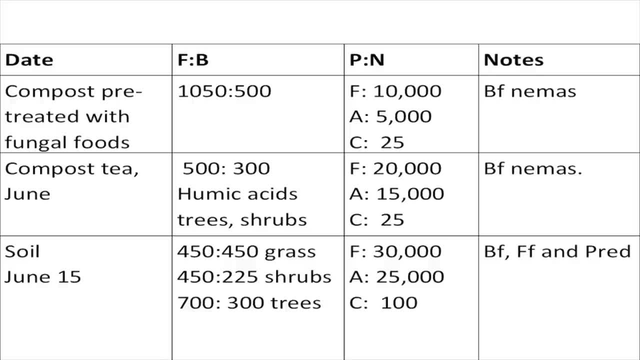 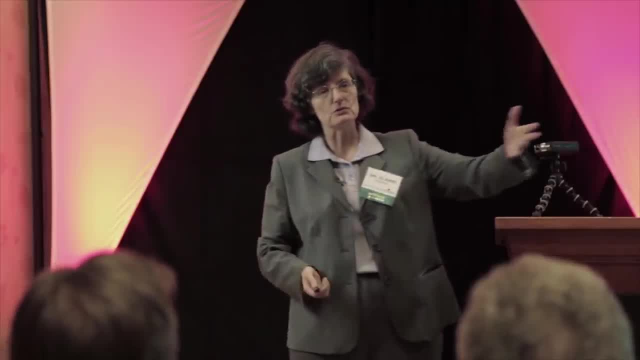 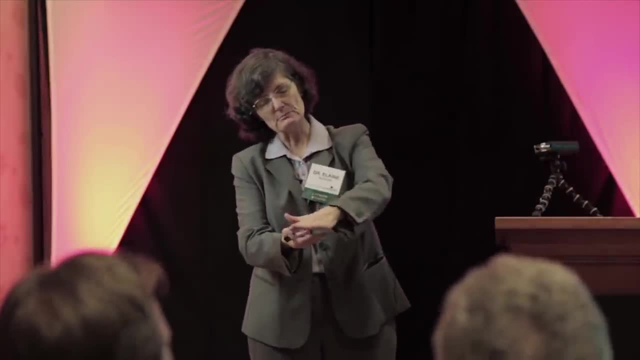 so you have to have tested your plant material before this and know that you've got these organisms sitting on the surface of that straw, on the surface of that dried plant material that you're happily storing. So that material just barely covered the bottom of the bucket And 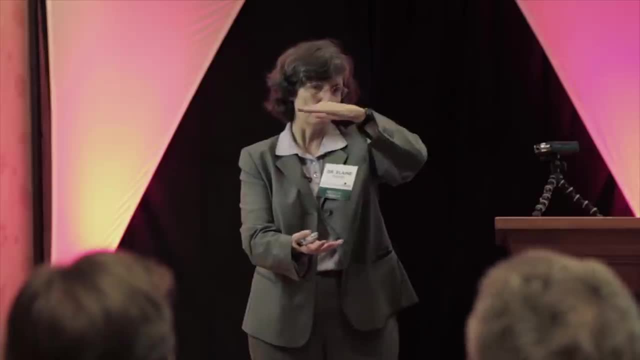 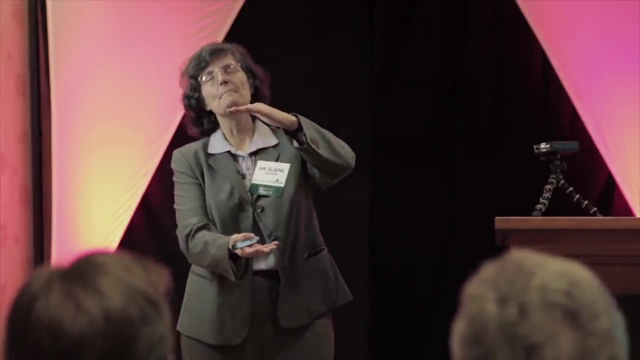 now you fill the bucket up with water- you know, not right to the top, but you know. So when you pick up your bucket and walk around, it doesn't slosh all over your shoes. So put water in there. Make sure that, if it's tap water, you have added a humic acid so that you get rid of the 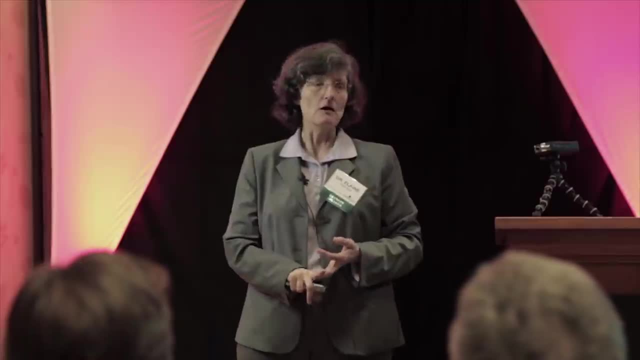 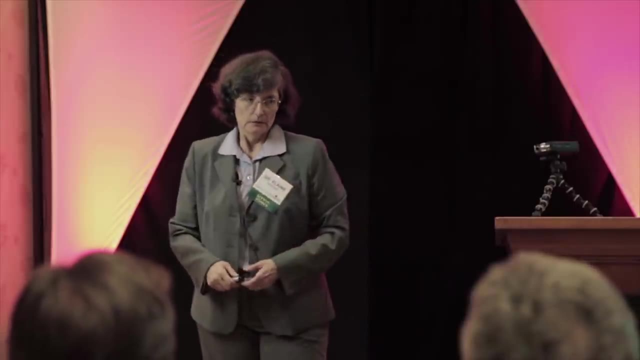 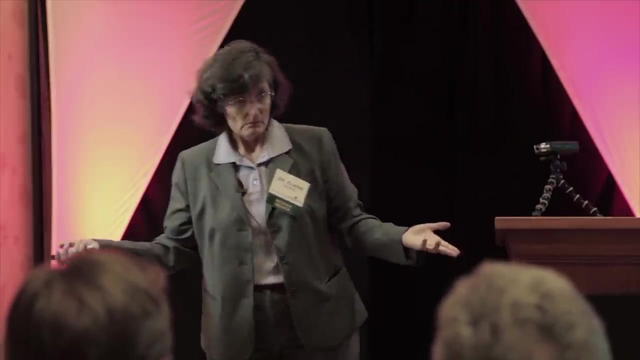 chlorine and the chloramine or any sulfur gases, any of the problem materials that might be in your tap water. Because why do we add chlorine to water? I guess what It works, You know. why do we put chloramine in? Because chlorine doesn't work very well anymore, because we've got a lot of nasty organisms in our piping systems, in the plumbing that they have to put chloramine in now to prevent the biofilm in the pipes when they're piping that water to your house. So what's the concentration of chlorine and what's the concentration of chloramine in your water? It depends on. 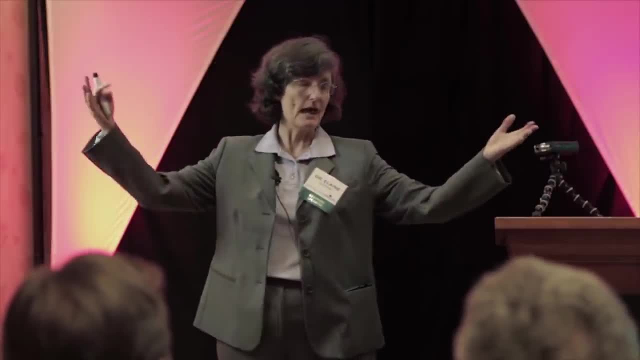 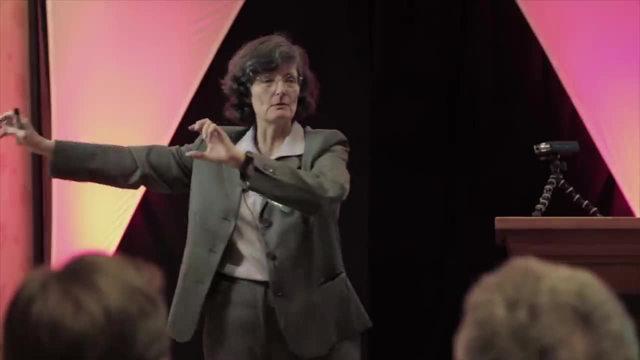 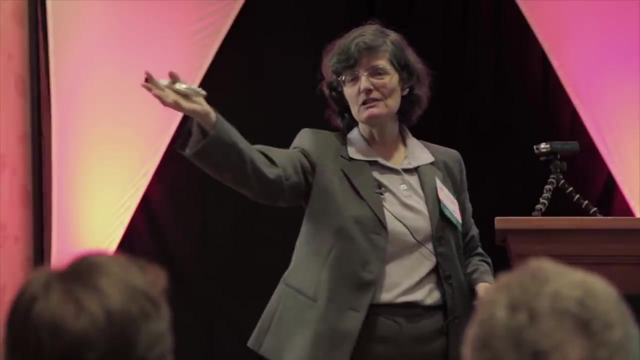 where you are on the pipes. If you're the last person on the pipe, don't worry. Chlorine, chloramine's gone. How many of you are the last people on your plumbing system coming from the water treatment plant? One, two, All the rest of you, How much chlorine and how much chloramine is in your water? 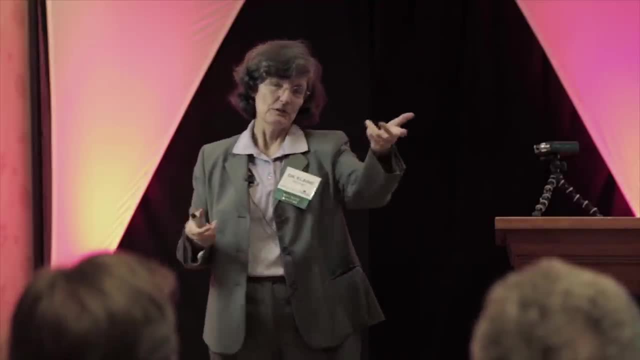 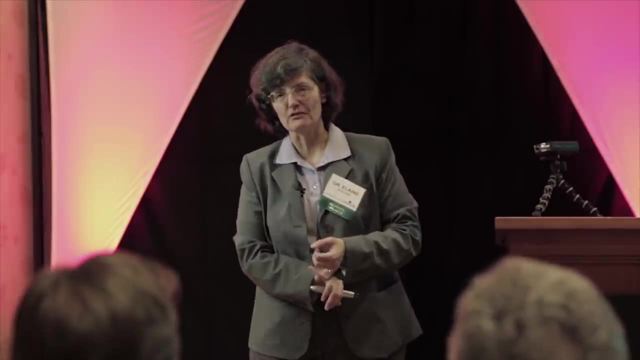 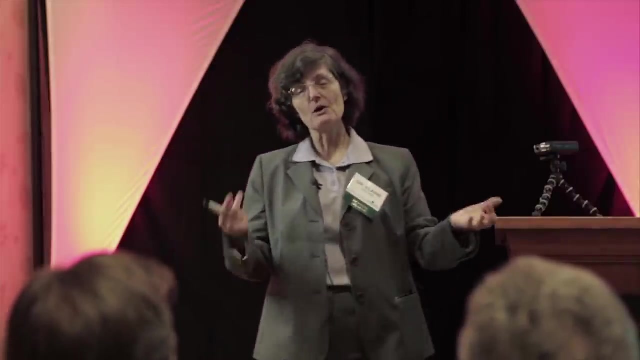 Well water, Well water. Do you have dissolved sulfur? Do you have other problems? How is your magnesium level? Oh, this part of the world, Magnesium, Manganese. You could have some problems. So let's kind of hedge our bets. Maybe you're not on tap water. Maybe you got a well water. When's the last time you tested it For excess nutrients of some kind That could be killing our organisms? So just hedge your bets. One drop of a good humic acid into a gallon of water and we've tied up. we've complexed all of these problem materials. We don't have to. 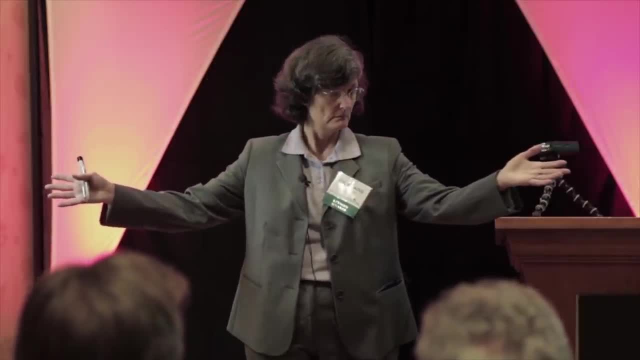 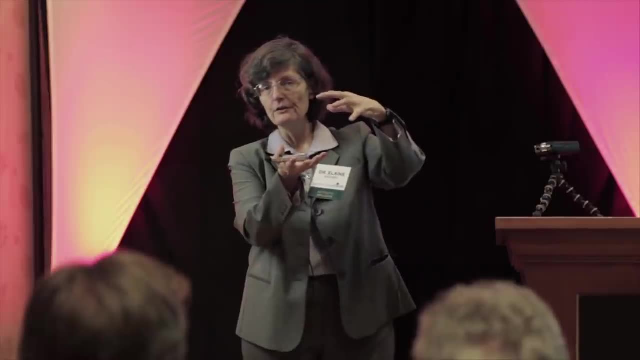 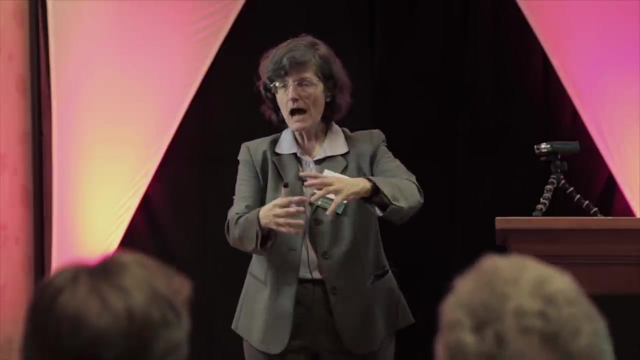 worry. Where are you going to get your humic acid? from Your compost pile. Take a couple cups of your compost, Stick it in a cheesecloth and a colander, Run four cups of water through there And, as that water comes out of the bottom, nice, deep, rich, dark brown color. What causes a nice, deep, rich, dark brown color? 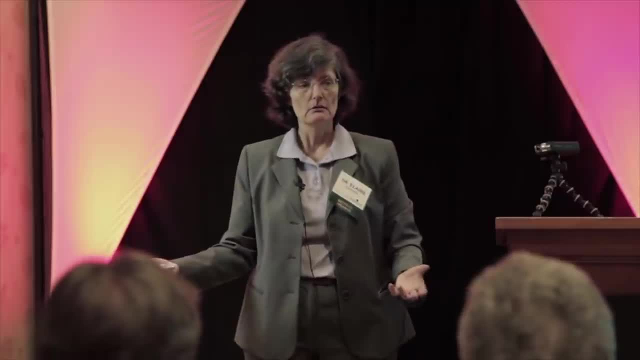 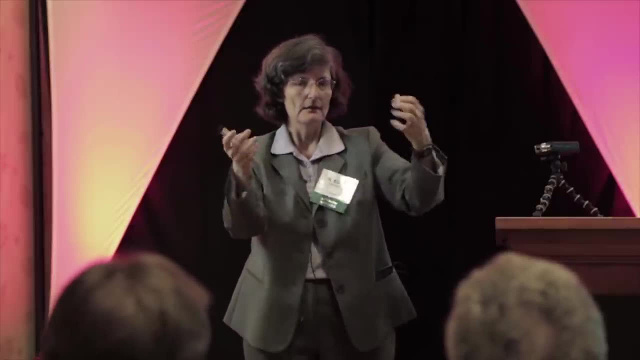 Humic acid. Humic acid, Make your own. So make a compost pile and extract it. Now it has to be passive. You don't want to be shaking, You don't want to be mixing, because that rips organisms off those surfaces and we don't want organisms. 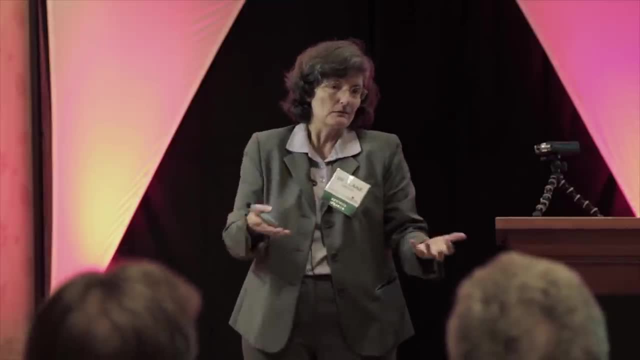 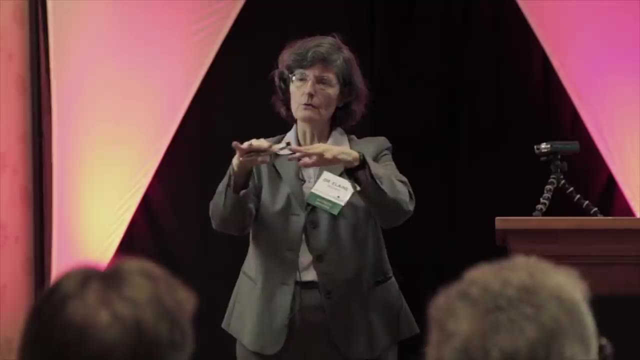 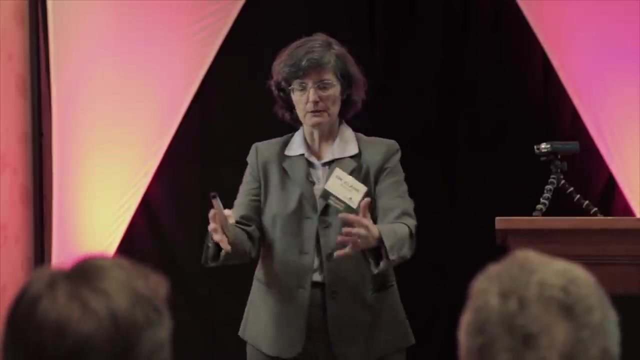 in our humic acid, Because they tend to eat the humic acid. So the humic acid's not left anymore. So passive movement of the water through that compost. Look at the color that comes out. Now take that first four cups and set it to the side. Put you in another container. Run another four cups of water through. Are you still? getting really good humic acid. Yes, Add the first two batches together and do another four cups. Now how much really good humic acid do you have in your compost? Is this super, duper outstanding compost? You're going to be able to run sixteen cups of water through two cups of compost And all of that will come out with really good. 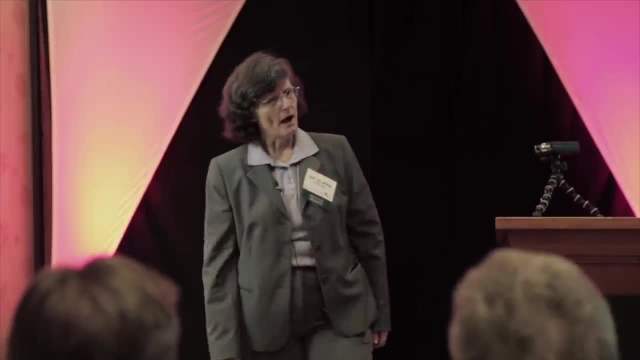 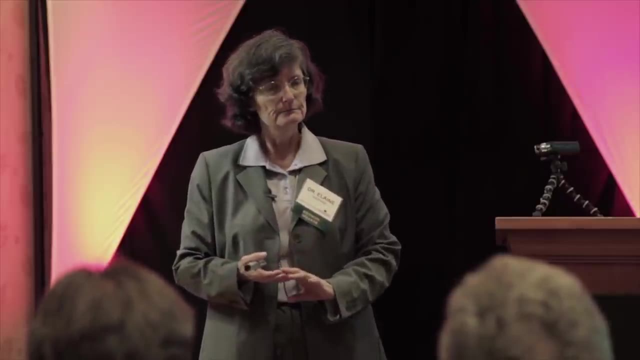 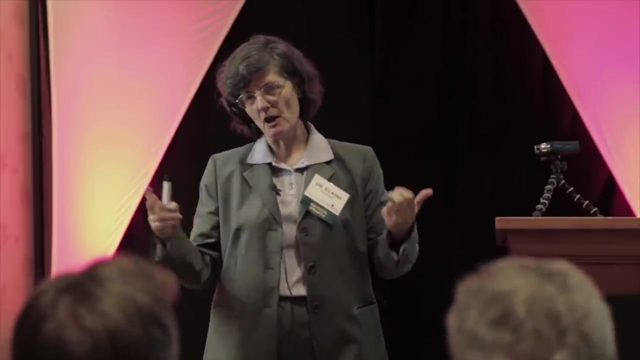 levels of humic acid. What am I using as a measurement? How do I know that I've got really good humic acids? Color Color. So where's the color Color chart? Do I have to go buy a Munsell color chart which costs several hundred dollars? No, Go to the grocery store. 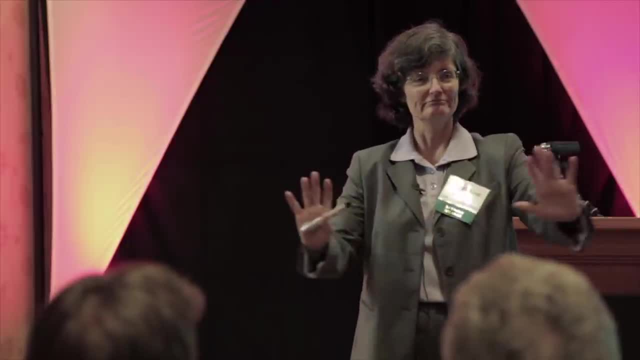 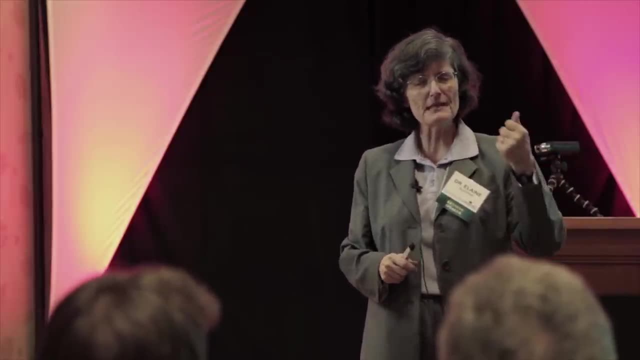 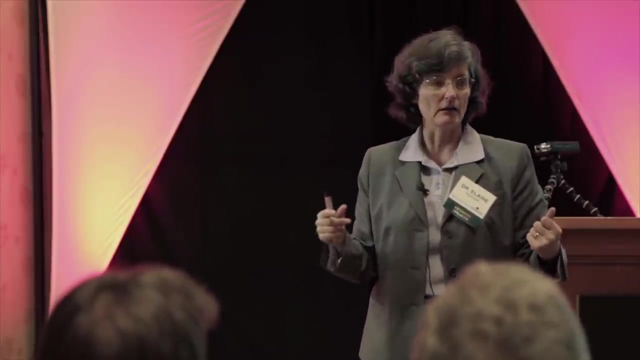 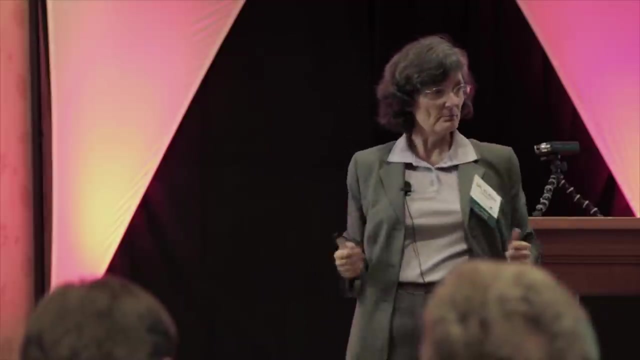 Go to the chocolate bar counter. Get a milk chocolate bar, because that's your fulvic acid color. Get a seventy percent cocoa chocolate bar. There's your humic acid color. So now you start running water through your compost. Do you have good compost? Pull your chocolate bars out. Compare the colors. 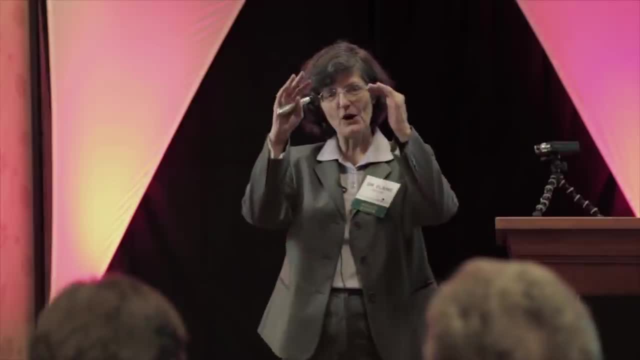 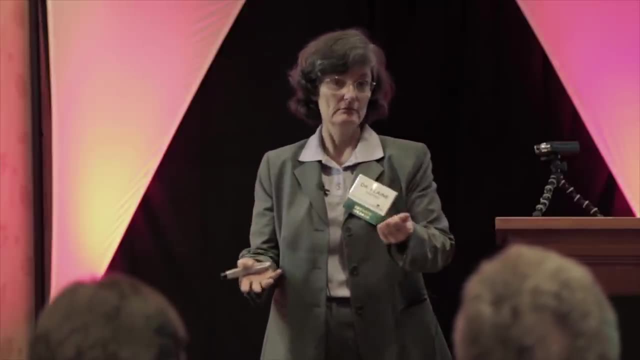 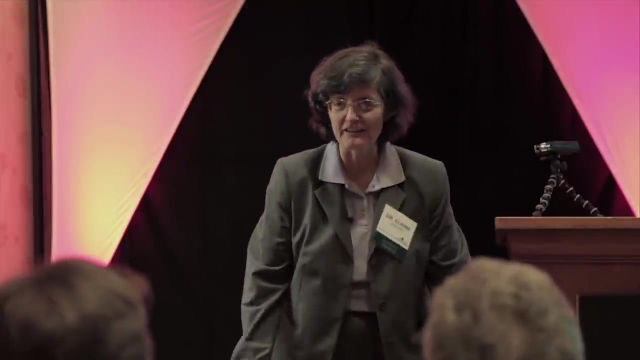 So if absolutely no humic acid is coming out of your- well, it's not compost- then at least you've got comfort food right there, Because you can always go replenish your color scale. Chocolate bars have not run out in my grocery store, So keep going. 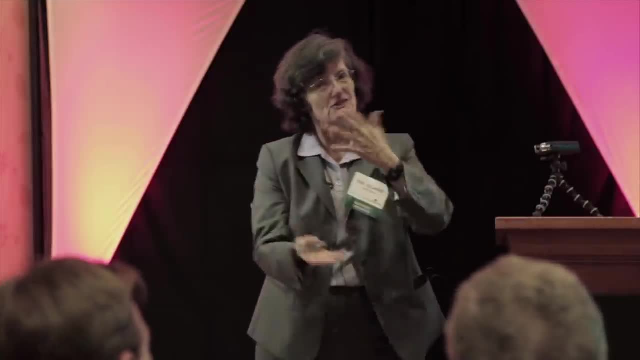 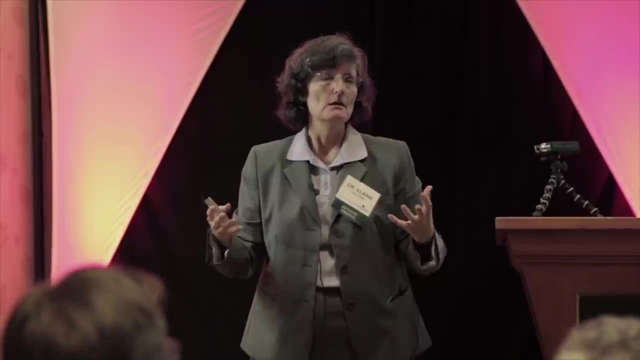 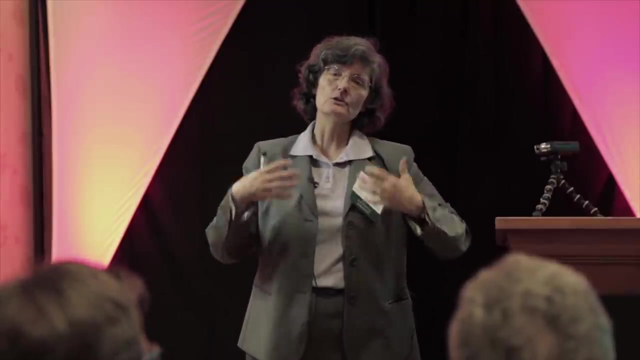 So protozoan infusion, I got distracted Humic acid in that water And now let that grow at ambient temperatures, Because the protozoa we want to be putting into our compost extract or our compost tea are those organisms that are going to survive under the conditions that are outside. 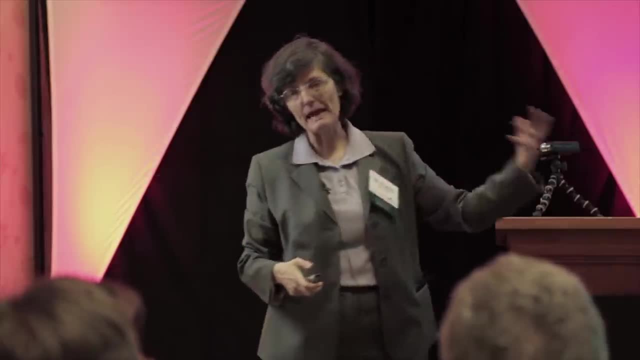 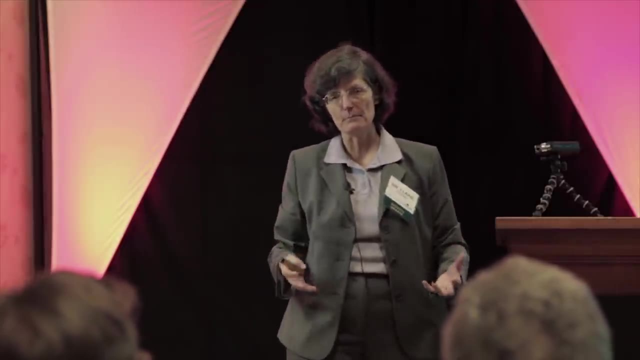 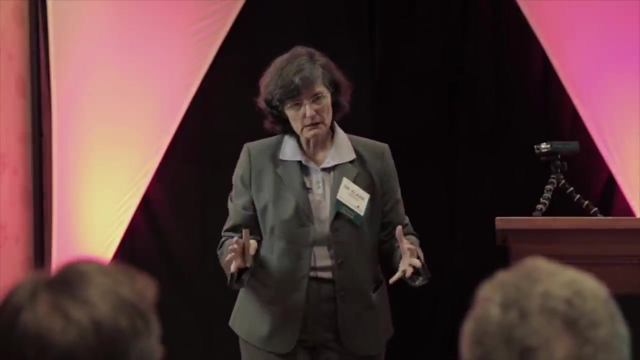 So whenever we're making tea, whenever we're making extract, whenever we're making a protozoan infusion, you grow these organisms At ambient temperatures. When I first started working with the Mirage Hotel in Las Vegas, we were very clear with them that the tea brewer had to be outside. 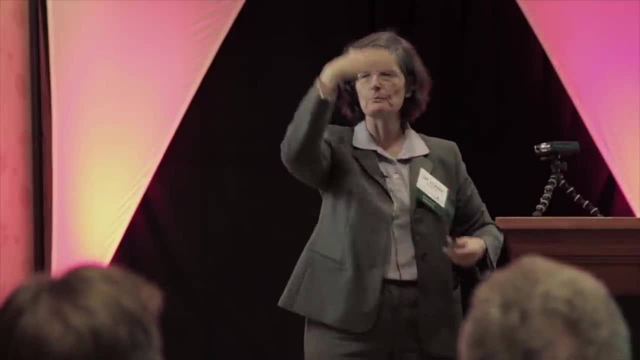 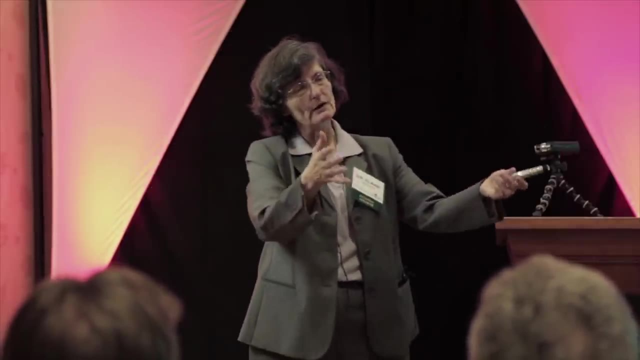 So we were growing those organisms. that when we sprayed them onto the palm trees, when we sprayed it onto the site caps, when we put that onto the lawn, Those were the organisms that were growing at that temperature. They were already used to 120 degrees. 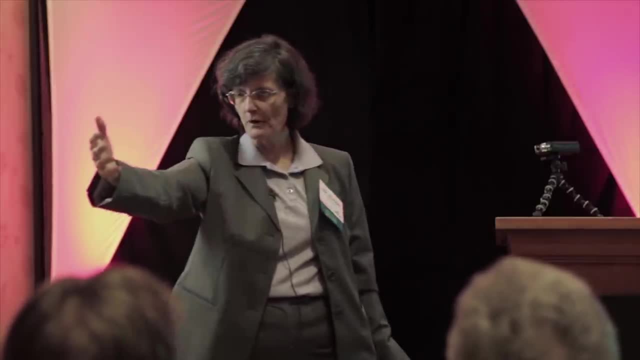 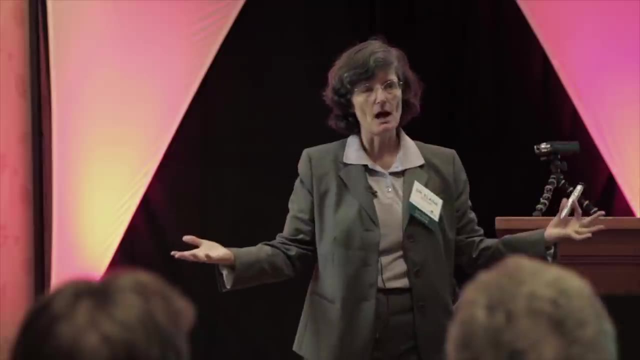 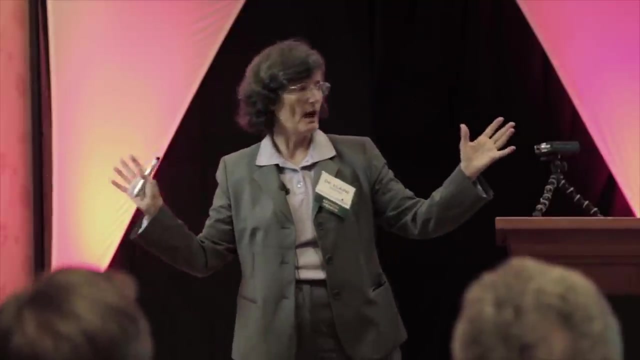 So there was no problem in getting excellent effects of applying these organisms out into the real world. Fantastic job on the palm trees. We got rid of all the fusarium, All the crown rot, Gone Very rapidly, All the dog spots, All the alcohol dumped on that lawn. Got rid of those spots. 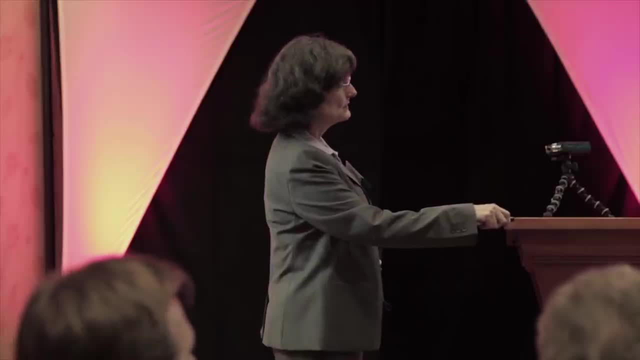 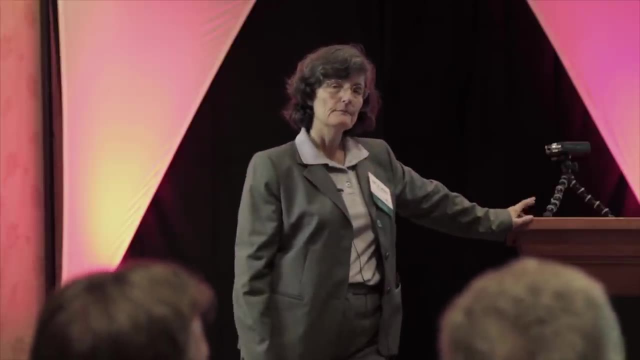 The end of May we went out there and did the soil. So two weeks after we put the tea out, Went in and looked at the biology in the soil. It's better, isn't it? But is it where we want it to be? No, 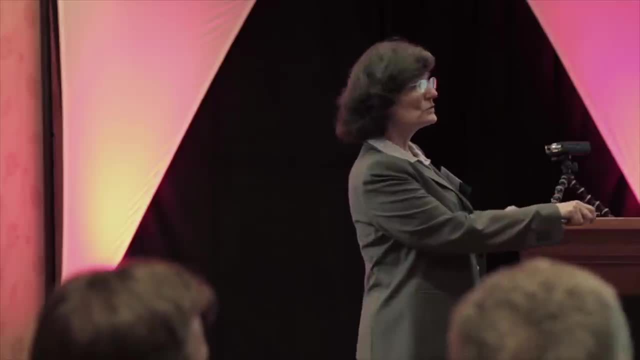 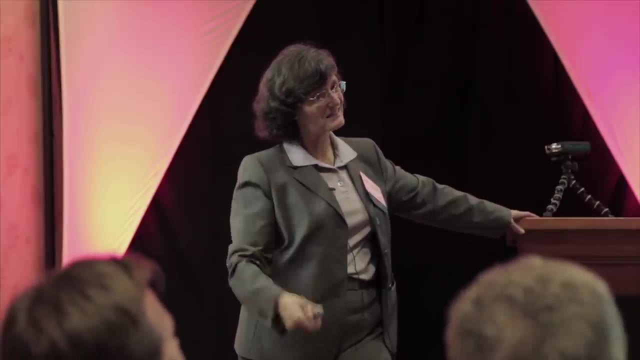 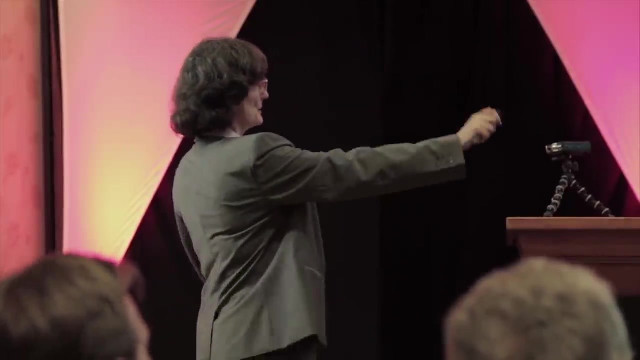 Well, at least we got the protozoa out there because we had the infusion, so we got good nutrient cycling. But we're still selecting for the not so wonderful species. Gotta keep going. Gonna have to do another one. So here we go, There we go. Here we are in June, And if we had really good compost last October, we wouldn't have to be doing all of this work. Okay, but we didn't get the organisms up and started, So, okay, let's do it again. But now our compost has had those good fungal foods in it for about a month and a half. 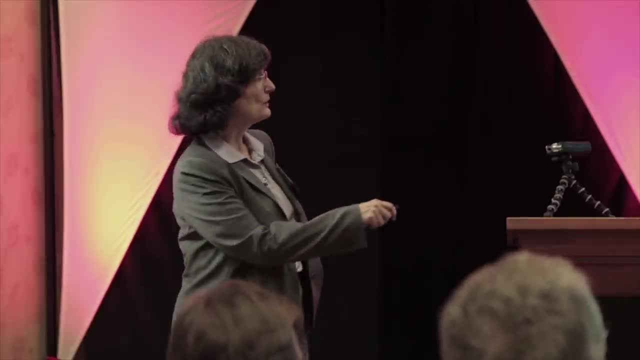 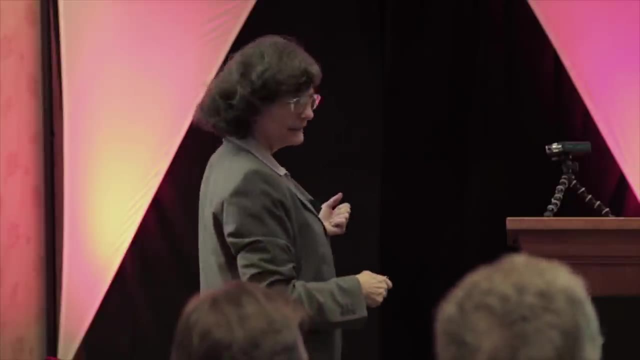 And look at what those fungal foods have done to our ratio of fungi to bacteria. Yes, We got it. We got our fungal community. Now have we fixed the tea brewer? Well, look at that, We do have fungal dominated tea. We're gonna add humic acids to that tea. where we put it down, around the trees, around the shrubs, around our perennials, We put in about half the amount of humic acid when we applied it to the lawn. We put no humic acids when we're going onto our veggies or onto our little flowers. 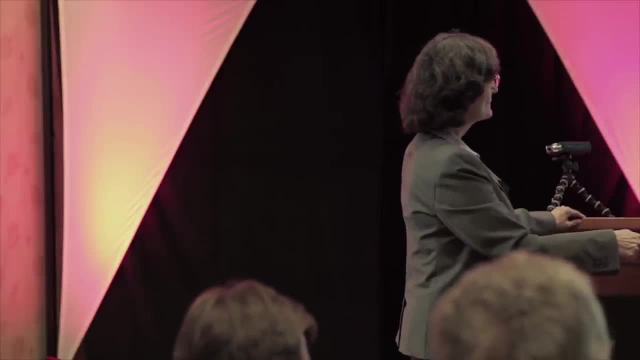 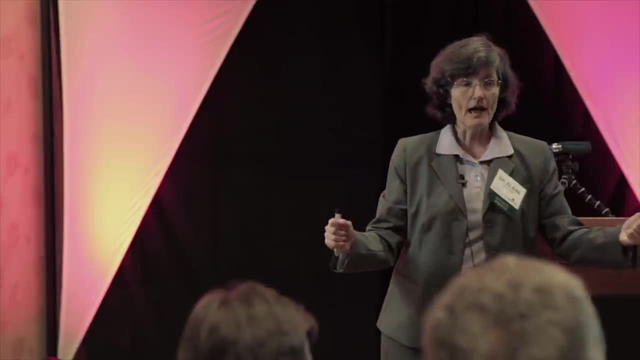 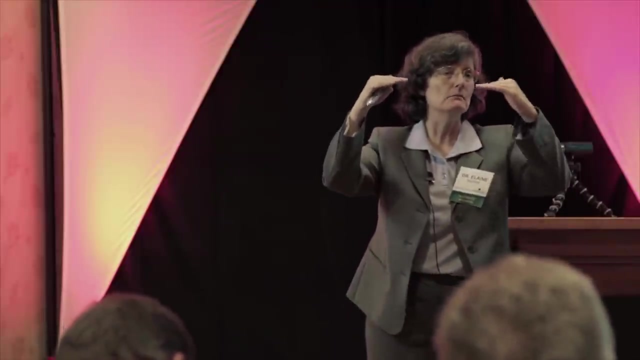 Good protozoa, good nematodes. Applied that out there. Early June, June 15th, we took another sample of the soil In the grass. Look, this is perfect: Equal biomass of fungi and bacteria and it's way above the minimum levels. 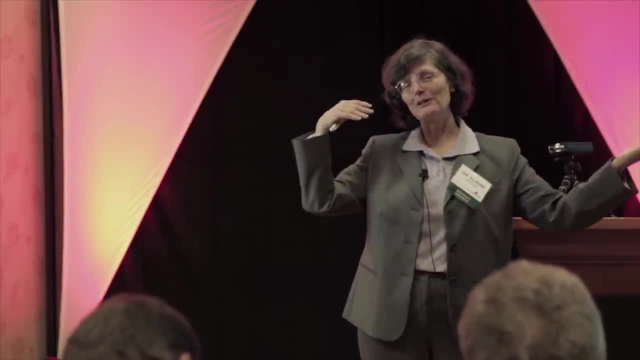 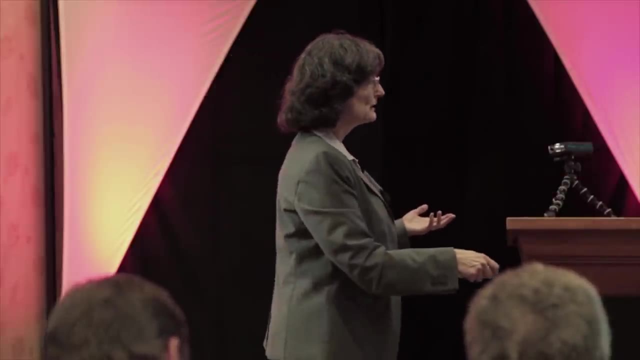 Whoa In our grass. Remember what it looked like come the end of September And we didn't have to use any water because we're building the structure. We got the nutrient cycling, We got bacterial feeding and fungal feeding and predatory nematodes. 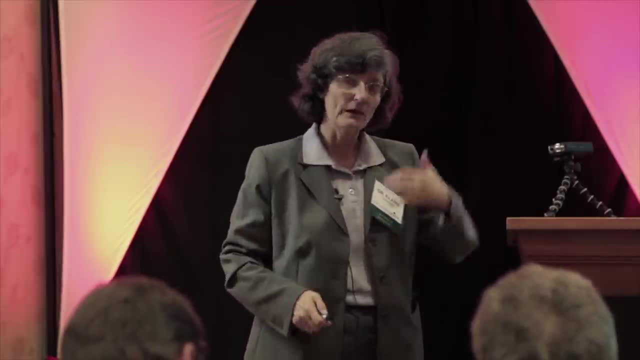 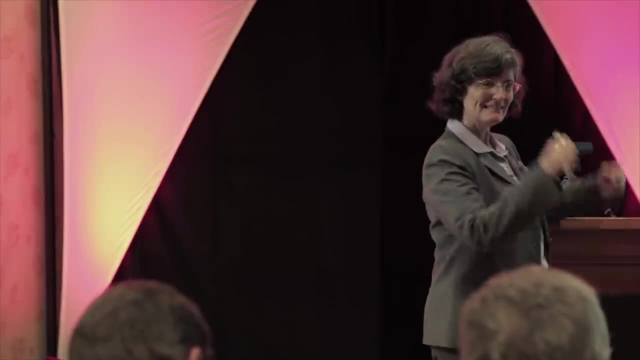 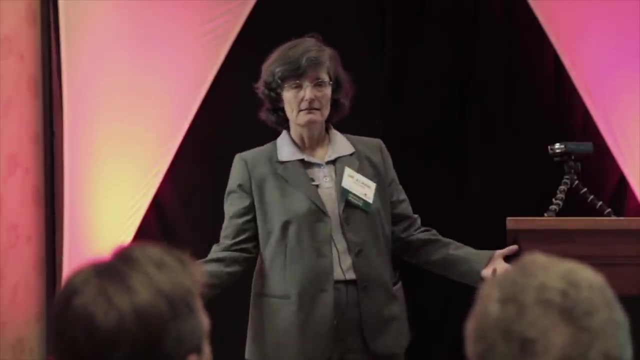 Came back into our lawn from September And we can document that they're there by we're looking through the microscope. Around our shrubs, Is that fungal dominated? Yes, Around our trees, Yes. So we managed to do it, But it took us nine months to get this conversion because we had people that 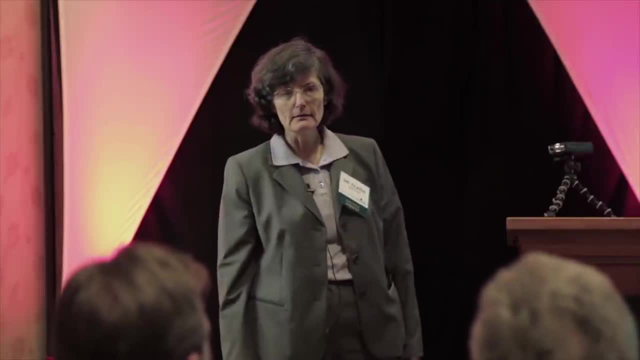 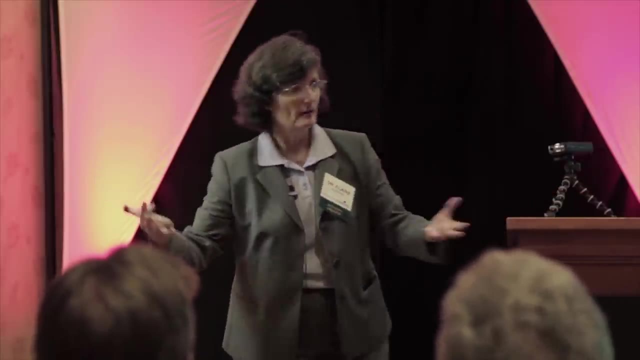 well, of course this is good compost. Yeah right, How do you know it's good compost Microscope? Learn how to use it. Or get somebody in your neighborhood, Now that you can come, you know, wander on over. 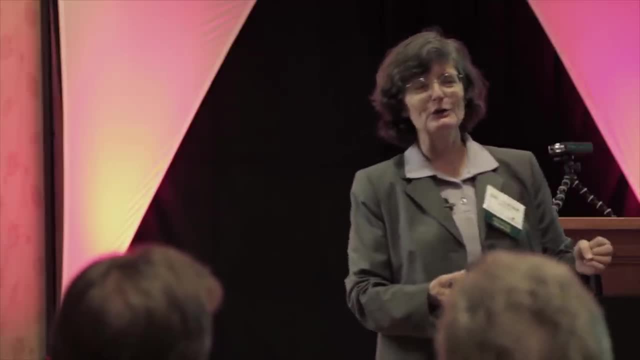 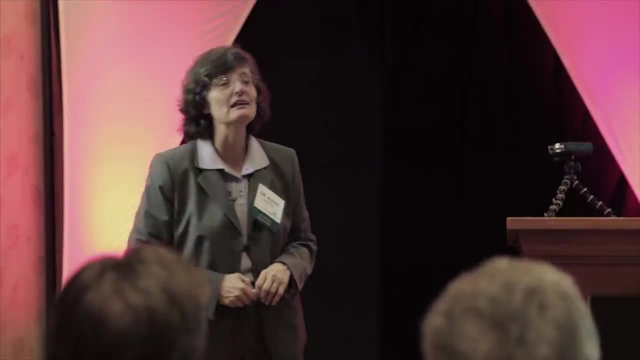 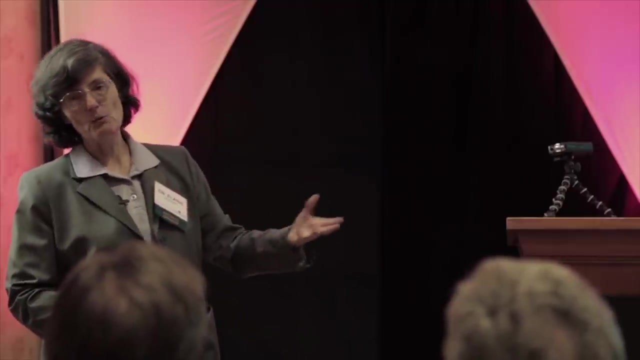 You're going to bring them a bribe, A little good coffee and a Danish And do my sample of compost or tea or extract or whatever you need. Get them to look at it for you, Because it's just, it's such a short process to look at any one particular sample. 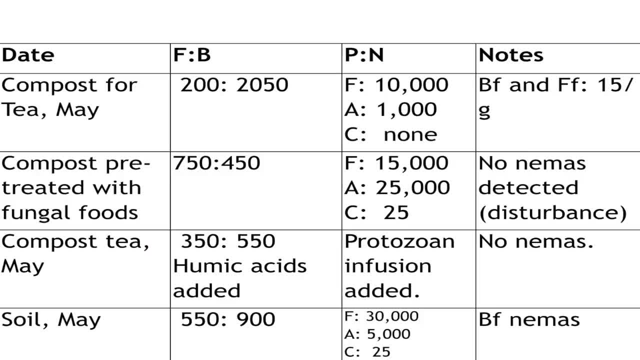 What is FAC? Oh, let's go back F flagellates, amoebae, ciliates, So three groups of protozoa. You know so really good aerobic protozoa. here A few ciliates, okay. 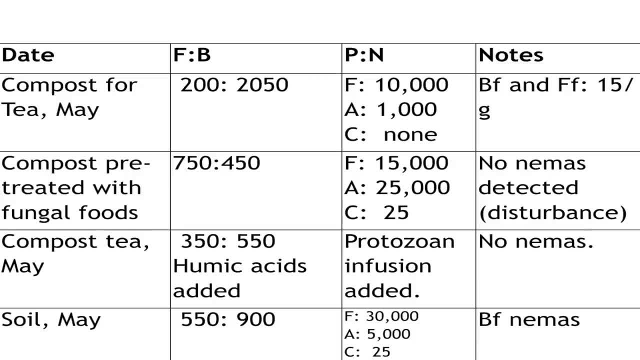 You're going to have some anaerobic microcytes. But you know, not bad enough As long as it's under 100 ciliates, I'm happy with it. So when you start going over 100 ciliates, 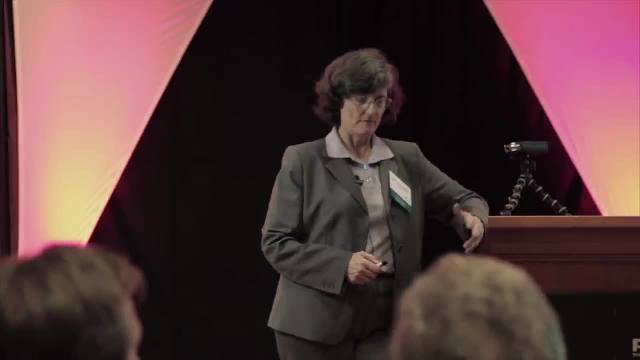 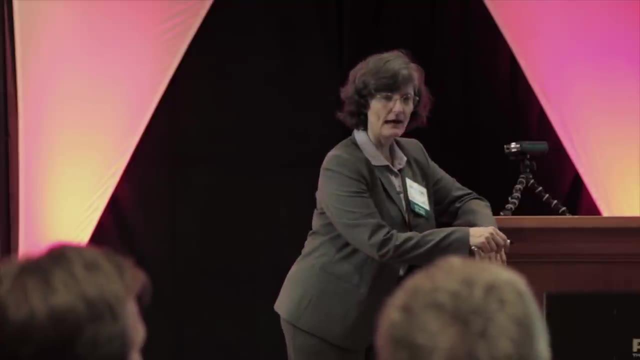 it's when you have more ciliates than you do flagellates and amoebae, That's when you're in trouble. So okay at 100.. If it started going over that, I'd know I had anaerobic conditions in my soils. 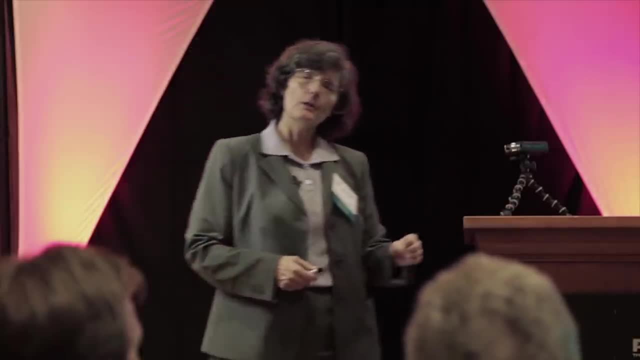 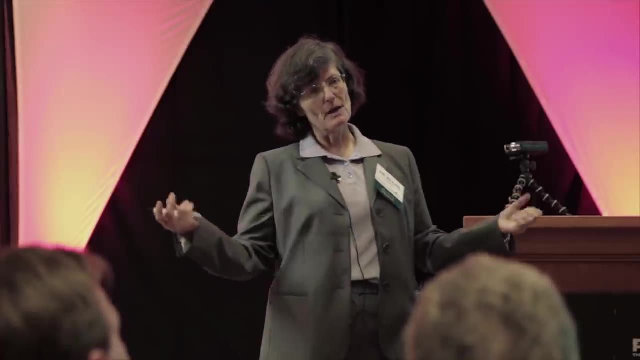 And I've got to work on that- Got to figure out where those are. How do you know where your compaction layer is in your soil? Penetrometer- And the penetrometer by any other name- is a metal rod with a pressure gauge on top of it. So go buy a metal rod. How expensive is that? 30 cents, Maybe $1.30 these days. Buy a little pressure gauge, Maybe $5.. And now put the metal rod- so the tip is on the surface of your soil where you want to test. 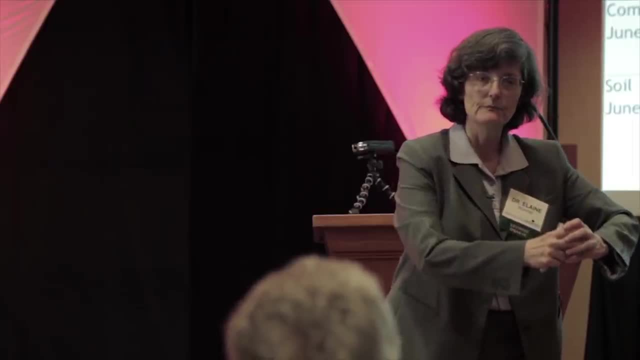 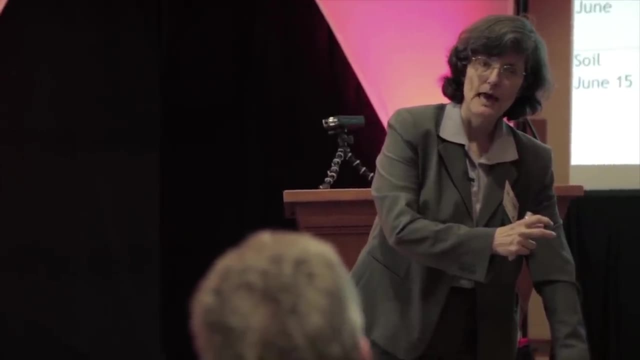 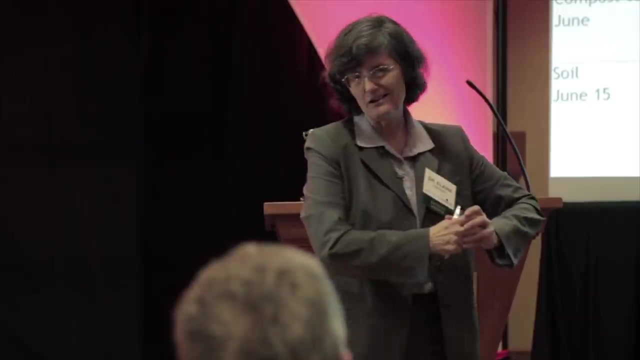 Your pressure gauge goes on top of that and start pushing And you can read the pressure that you've got to be pushing to get that metal rod to go into the soil. And if you go above 150 psi, pounds per square inch, if you're pushing harder than 150 psi. most of the roots of your plants cannot move through that soil. It's too compacted, It's going anaerobic. Those are not happy campers. You're losing your root systems at that depth. Now we've got some plants that do tap roots. 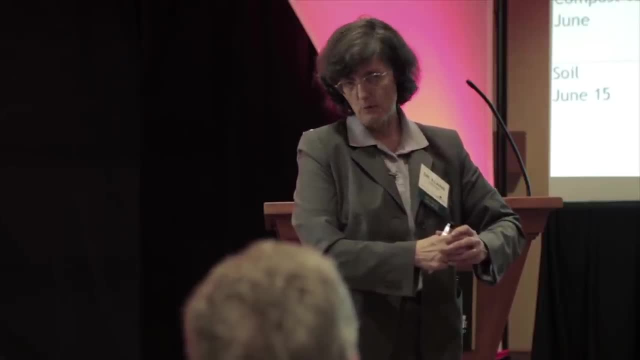 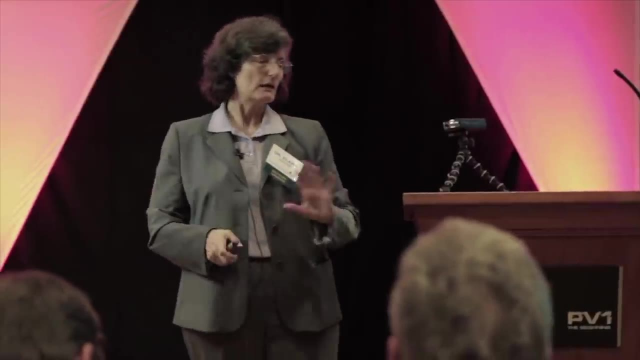 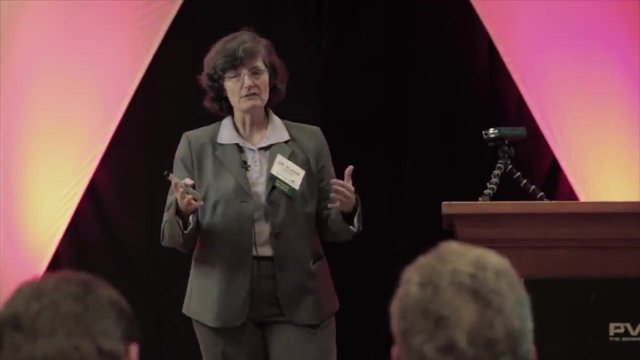 So if you've got some tap rooted plants, they will be able to push that tap root into the soil up to 300 psi. So there's a couple of interesting publications from Pennsylvania State University, Penn State, Where they have documented all of this kind of information. What's the compaction as measured by psi that stops roots of different kinds of plants, And any time you go over 300 psi, roots cannot push their way through that at all. And really is it the density of that soil that's a problem. 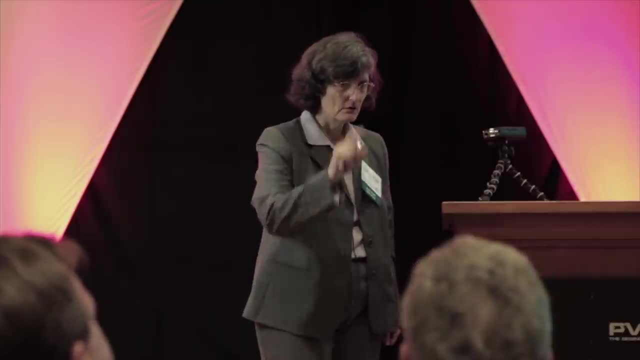 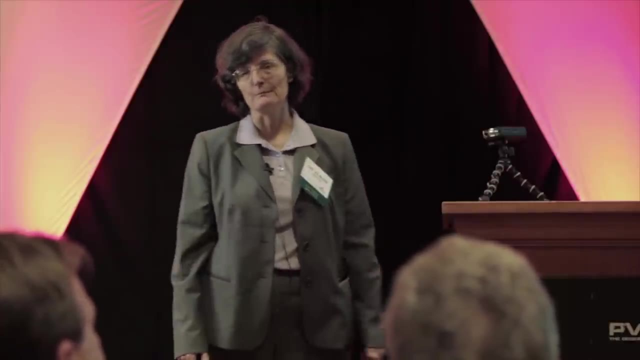 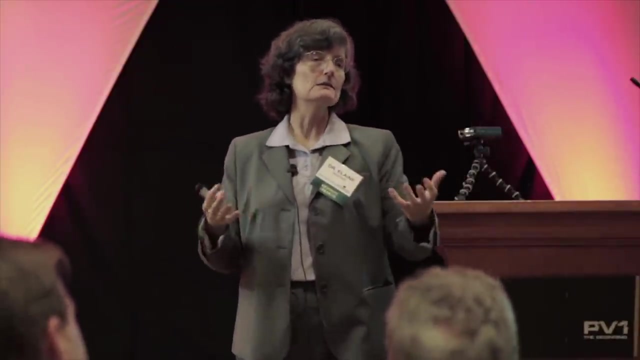 Or is it the fact you're going anaerobic Bingo Because your roots can push their way through Concrete. So why would a little bit of dense soil be a problem? Because you have no oxygen. So he's asking: what are some of the other characteristics that we could be looking for instead of using a microscope? 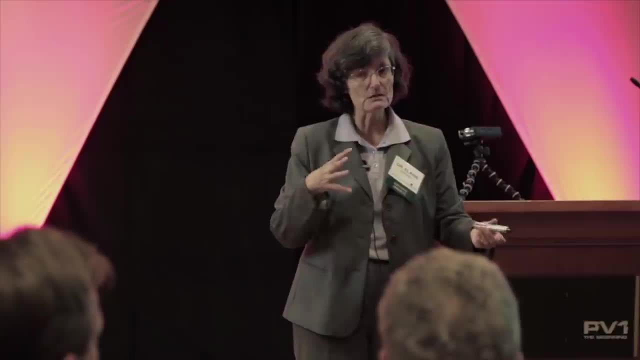 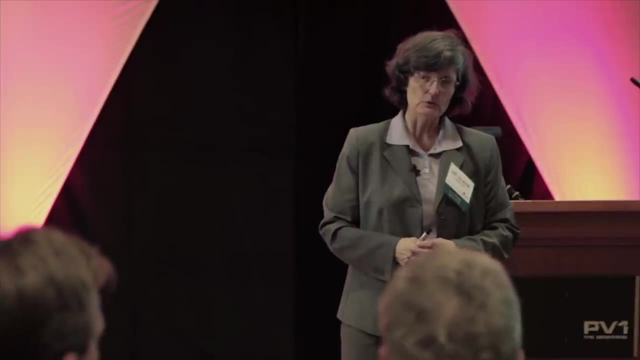 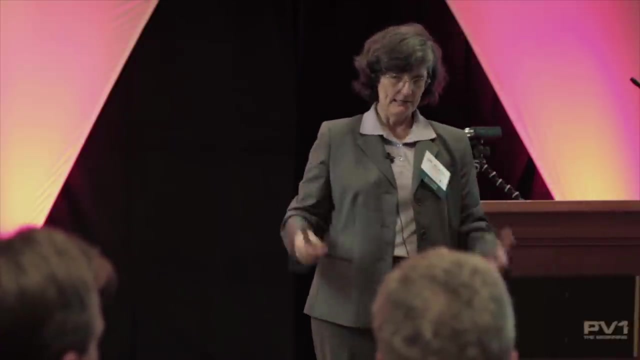 It's really hard to interpret other characteristics, And when I do the two or three day course Life in the Soil, I go through a lot of those other characteristics And I always want to give the explanation for why, And so I need another 48 hours to answer that question. 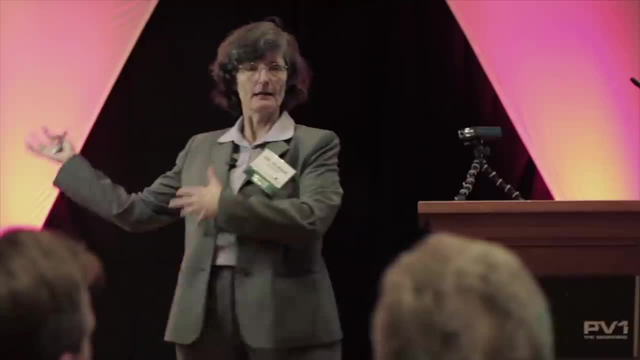 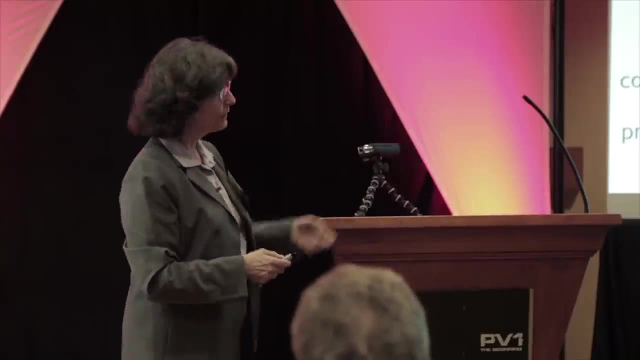 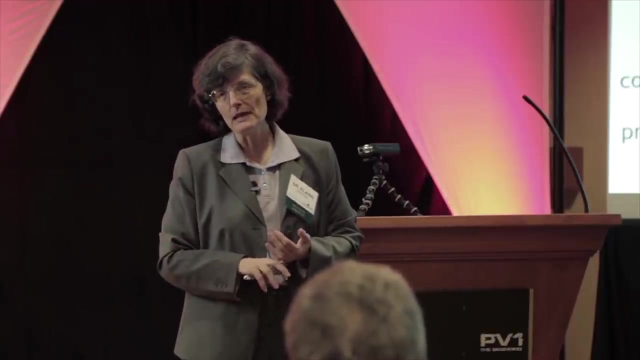 So come to the seminar next week and I can go through all of that Question. So, just like this example that we went through, first thing that you want to do is take the before picture please, Because I'm always amazed that when we go into some farmer's field, when we start working with clients, we're there with it's weeds. We got weed city Annual problems. The grass that's grown is bromus or Bermuda grass, And they've been told that the only thing that they can grow anymore is Bermuda grass in these pastures. There's no nutrients, You have no ability to hold water, So the only thing that you can grow is Bermuda grass. How many of you have actually ever tried to keep a cow alive on Bermuda grass? Ain't happening, is it Not too good? 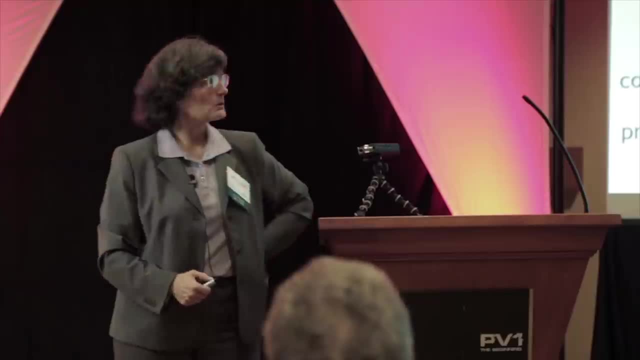 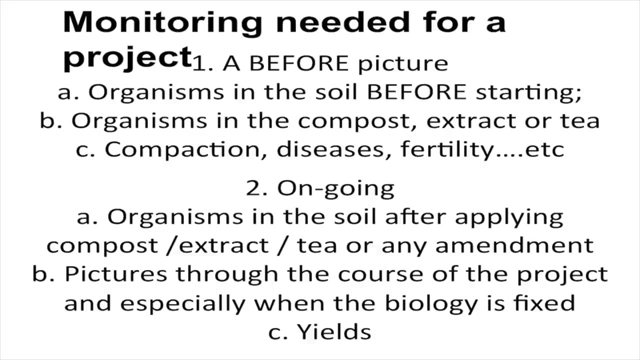 So we want to shift that species. So we want to take some really good compost, We want to get those organisms. So look at your compost. What are the organisms in your compost? Is it easiest for you to spread compost? So now that's up to you. 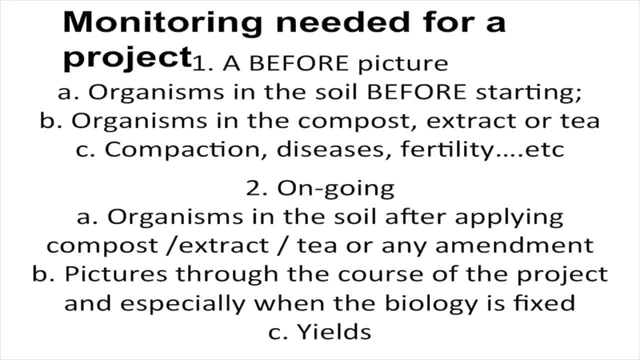 You know I can't tell you If you've got the equipment to spread compost, if you're making enough compost, you've got access to enough, really good compost with the proper sets of biologists. Then put the compost out, Because not only are you putting the organisms in the soluble nutrients, 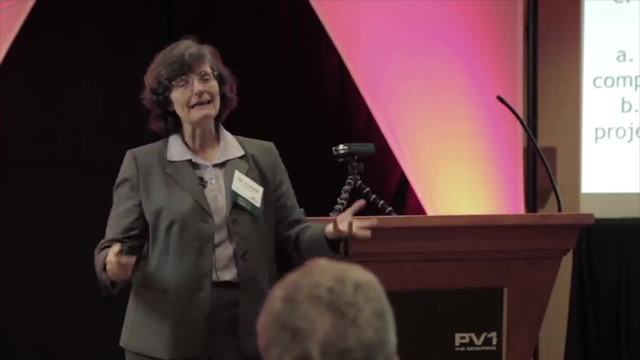 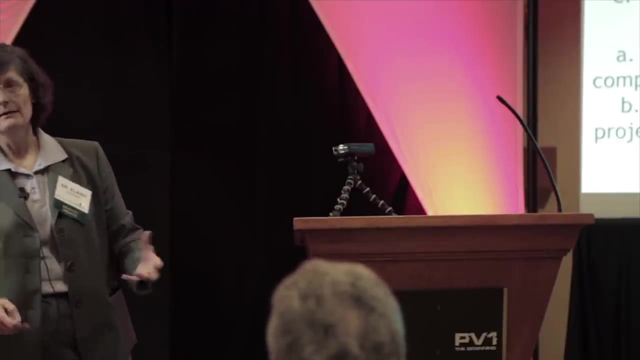 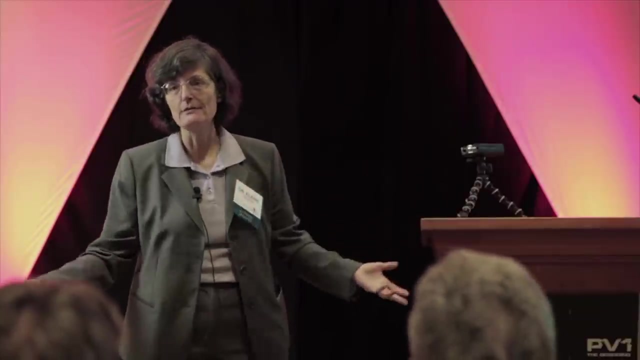 but you're putting the not soluble nutrients, the good organic matter. So, if possible, I will always choose to put compost out. But you know you've got 10,000 acres of range. How are you going to get 10,000 tons of compost? Because typically we're putting compost. if that's what we're doing, it's one ton per acre. It's an inoculum. You've got to make sure that you've got plants growing, that you've got food to feed those organisms. 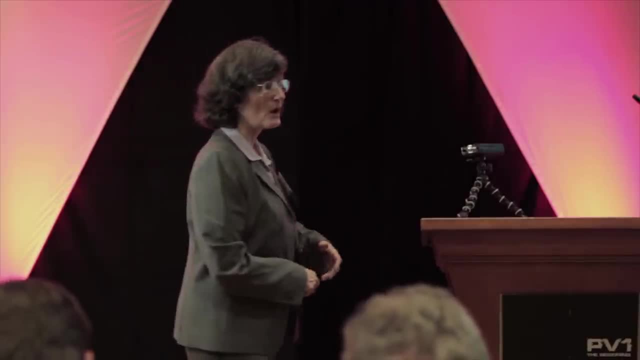 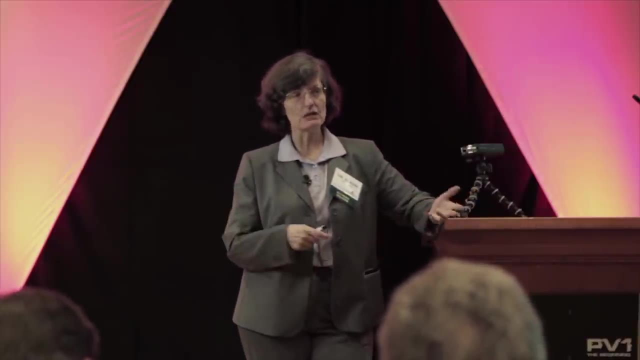 Maybe you add some humics, Maybe you add some fish hydrolysate, But if I'm putting compost out bare minimum as long as we've got the good biology, and I would probably be putting it out with food, depending on what did we find before. 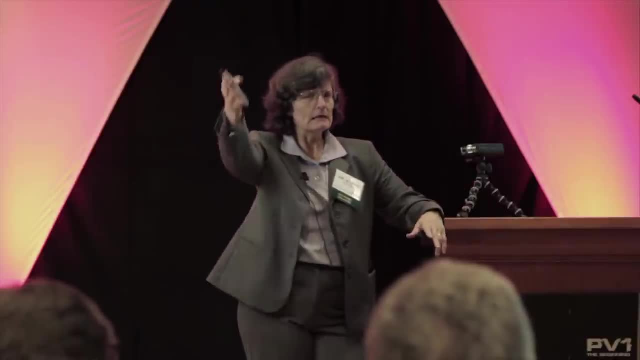 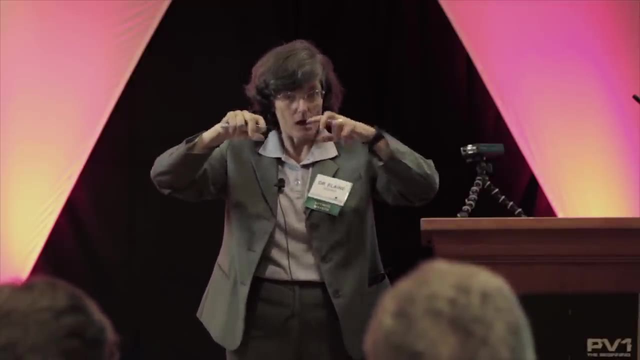 So I've got to walk your land, I've got to work with you. Do we need to put swales in? Do we need to put water holding? Do we need to slow down that water as it's moving across your property? Well, okay. 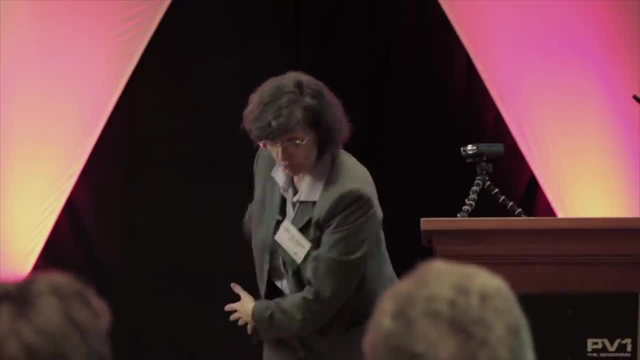 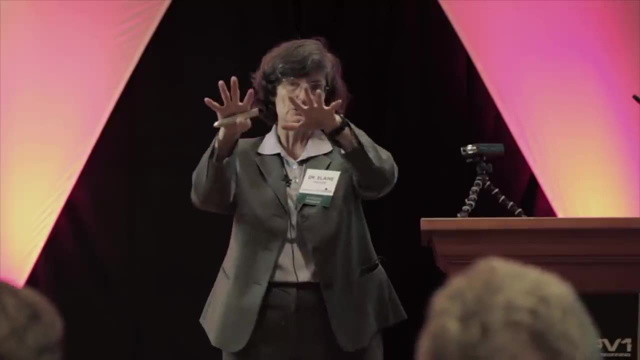 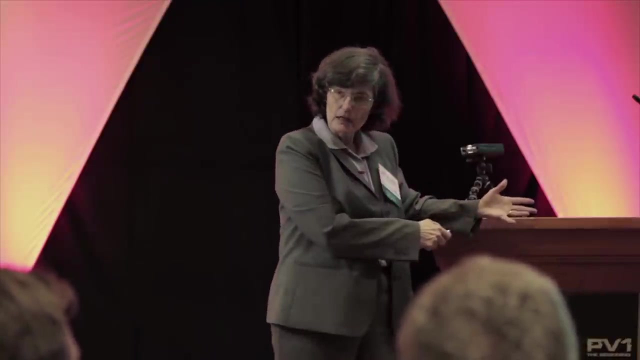 We better be out there looking at all these things, because if your water is going, It's going to take too long to get the biology established properly to shut that down. So let's do the permaculture thing. So maybe you don't have a lot of compost. So Maybe the extract is going to be easier. You've got enough compost that you can be using five pounds of compost per ten gallons of your extract water to get the biology extracted from the compost and into that water and apply that out and get the response that we want to see. 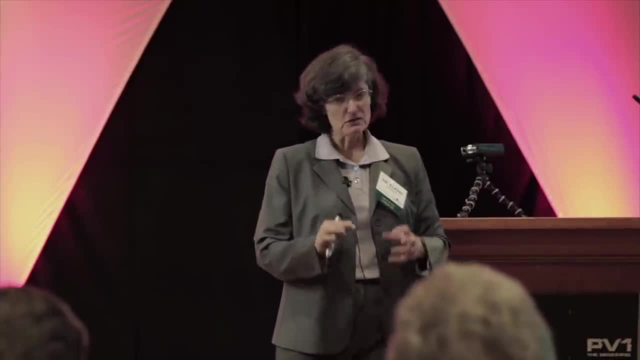 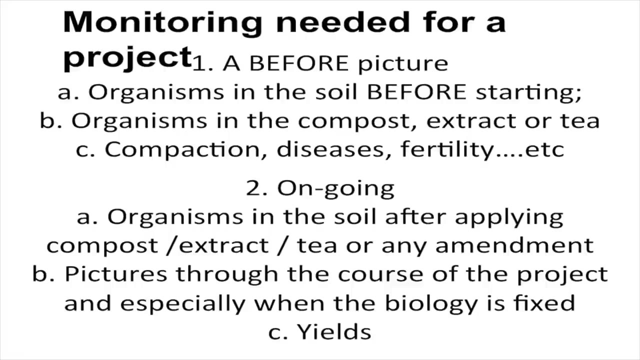 Maybe you don't have very much compost at all. You have just a teeny tiny small amount of really good compost. So now you're going to make tea, Because we multiply the organisms by adding food. Step one in a tea is to extract the organisms into the water. And we're adding foods then to get them to grow. Bacteria typically multiply every 20 minutes in a compost tea, as long as those are the ones that can grow at that temperature with those nutrient concentrations, yada, yada. So they're going to multiply by a million-fold overnight. 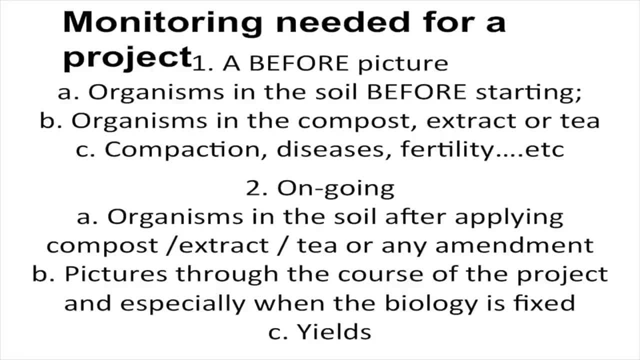 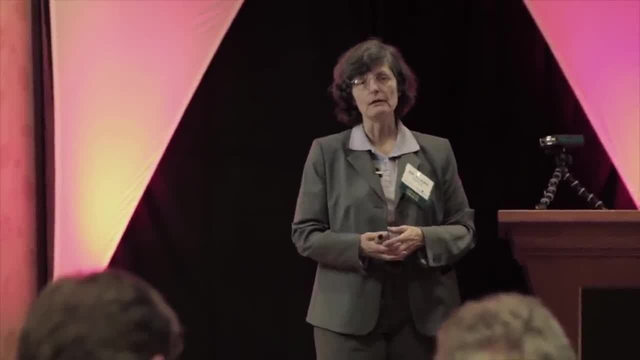 Fungi. Fungi multiply every four to six hours, So we're going to increase the amount of your fungal biomass by a hundred-fold overnight. Protozoa will multiply three-fold in a 24-hour period. Nematodes- I'm sorry it's too short a time. 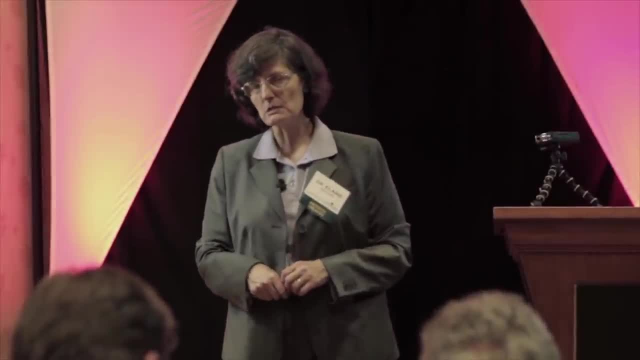 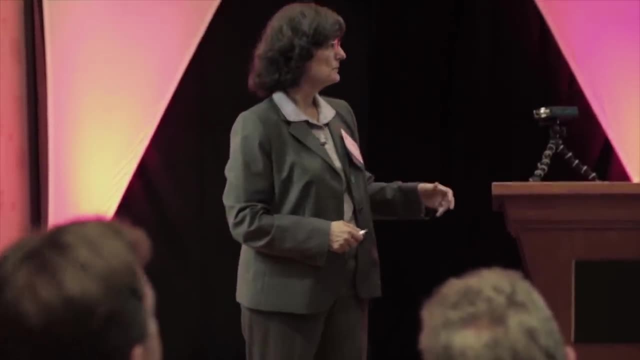 They cannot multiply in a compost extract or a compost tea. So whatever nematodes are in your compost, it's going to be in your extract or your tea. So are we getting enough? Typically, if we're going onto soil, I am not ever going to use tea on soil. 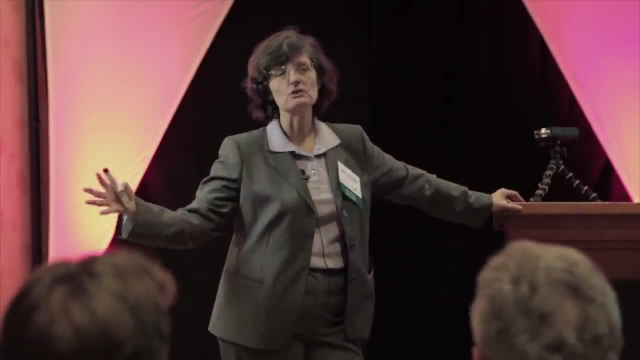 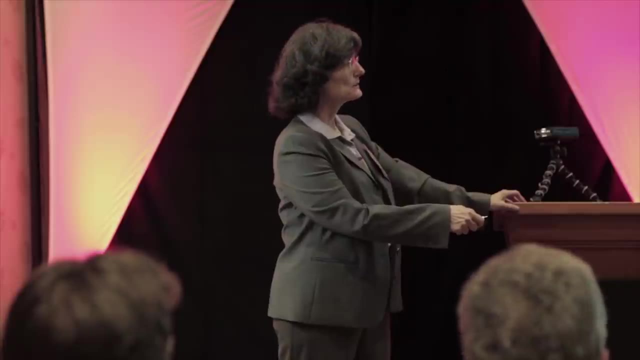 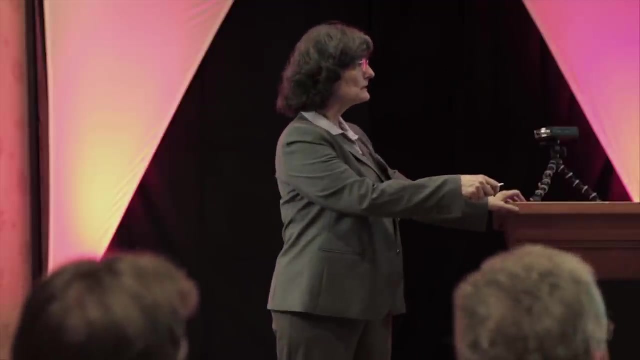 unless I just don't have very much good compost at all. So we're going to be using five times less compost to make a tea as compared to an extract. So got to know what the biology is in your compost to know how much compost you're actually going to have to use. 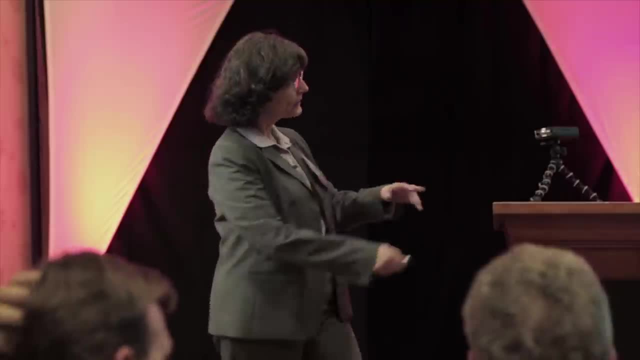 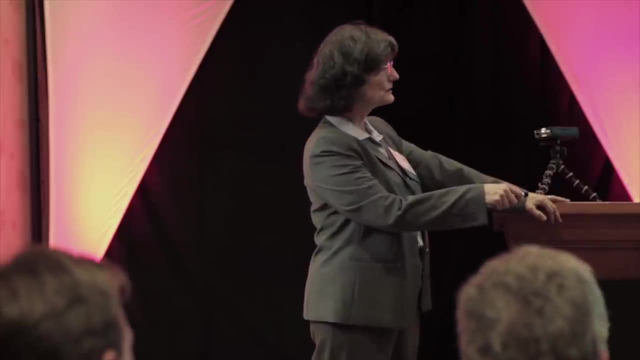 in making an extract or making a tea. So now I'm going to put that out. I want to be paying attention to where was the compaction? What were the diseases we had in the past? What's the fertility problems? What are the insect pests? Get some history on that. And then did we fix those problems. So be measuring that over time. If we come back two weeks later after applying this, we are going to, two weeks later, measure the soil. Did you get the organisms up to where they want to be? 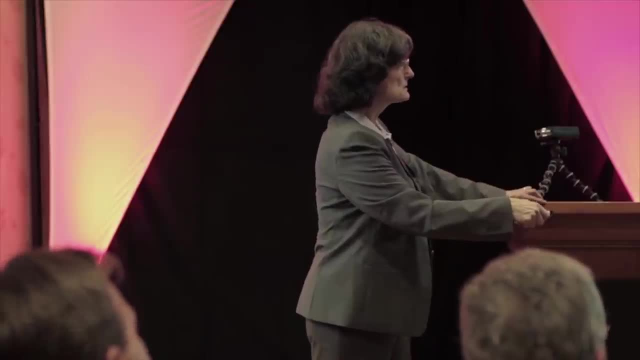 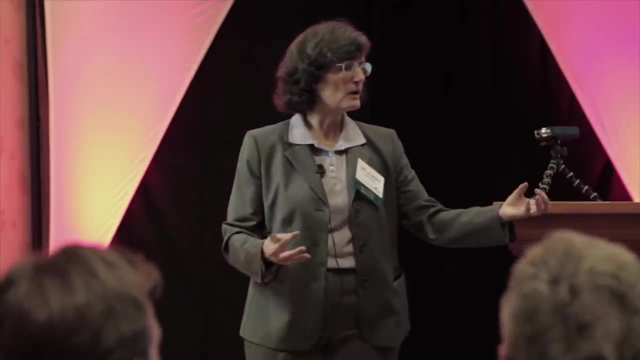 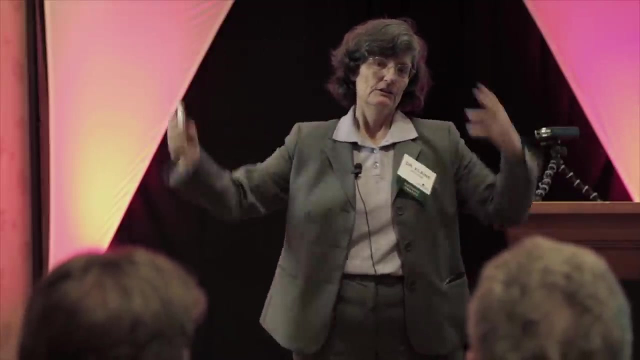 If not, then you're going to repeat. Please take pictures through the course of your remediation So at the end of the year, when you have an absolutely beautiful pasture of blue grandma or black grandma, you can take your client out there and say: 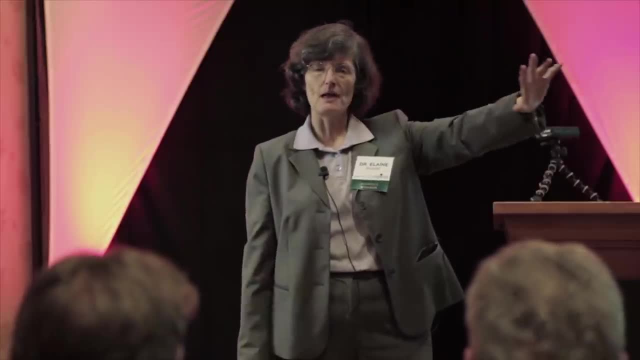 see, look at what we did, And when the client goes: oh, that's what we did, That's how this pasture has always been. 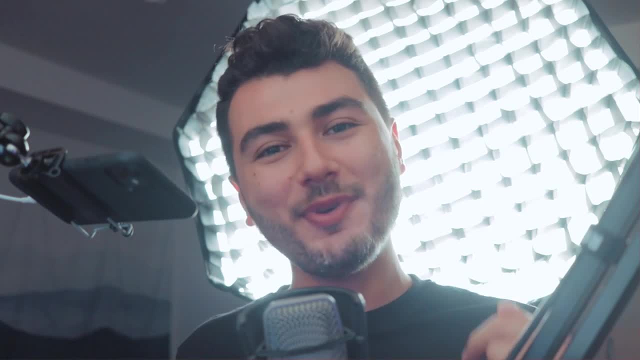 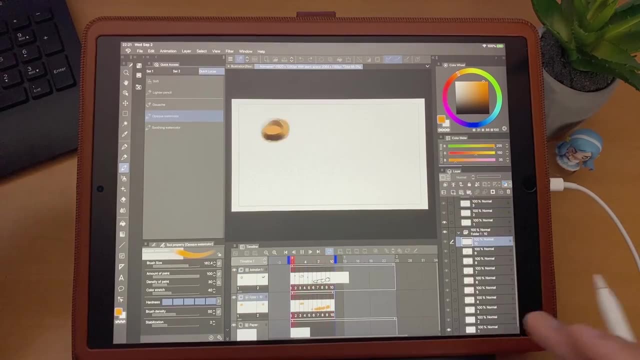 This video is sponsored by Paperlike. Today, I'm gonna be sharing with you five of the best animation apps available for the iPad. After watching this video, you will know which app is right for you If you want to make coloring easy. recording audio for your animations.